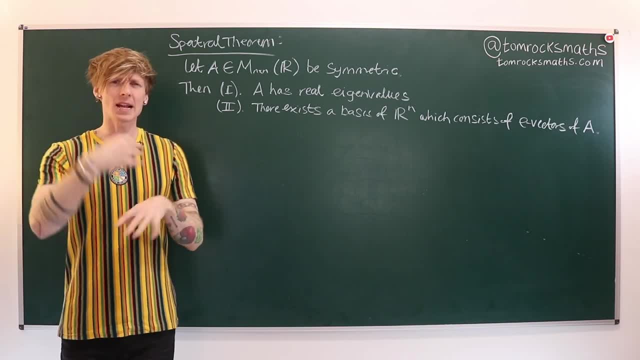 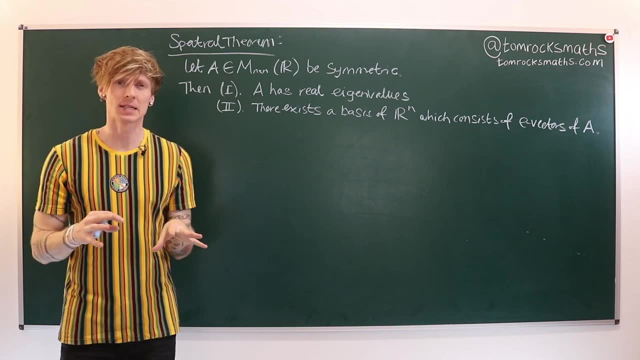 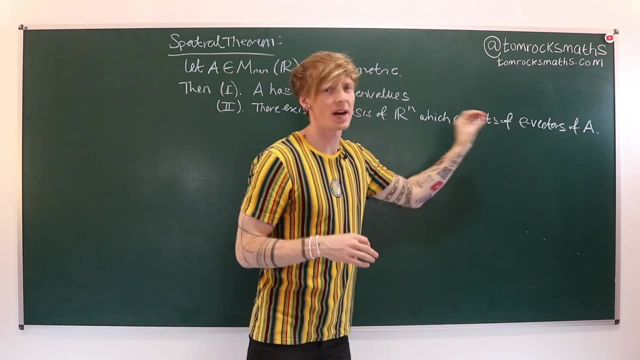 is such a big result and it actually comes from how you use it to diagonalize matrices, so how it's used in practice. Because once you know that there is a basis of your vector space consisting of eigenvectors, then that means there exists a similarity transformation. 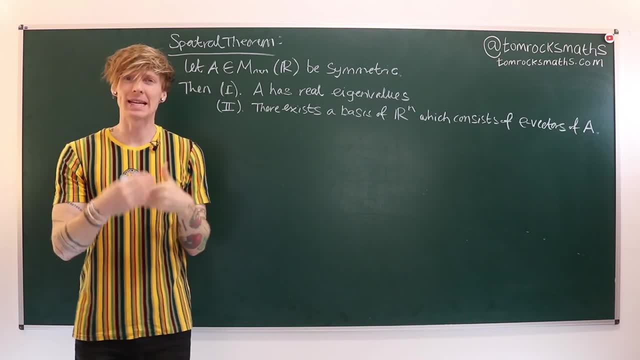 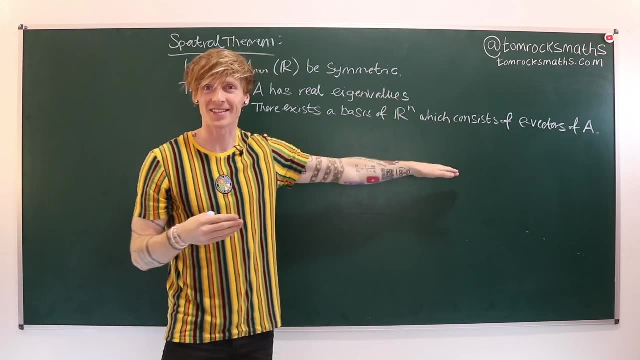 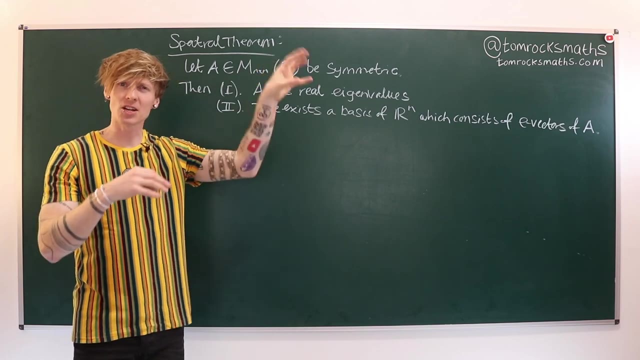 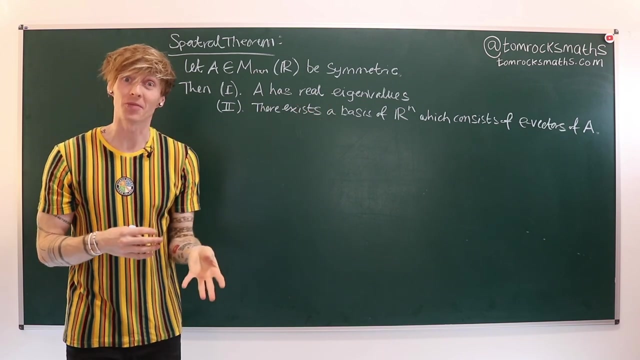 to turn your matrix A into a diagonal matrix, and you do this by changing basis to the basis of eigenvectors. So once you make that change, your matrix is not only diagonal but the entries along that diagonal are exactly the eigenvalues. So it's incredibly helpful because, as anyone who has ever worked with matrices will tell you, 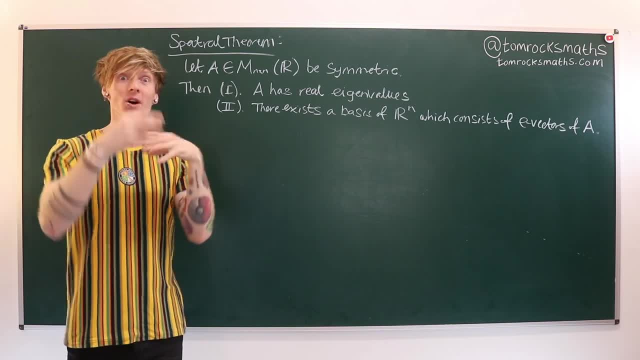 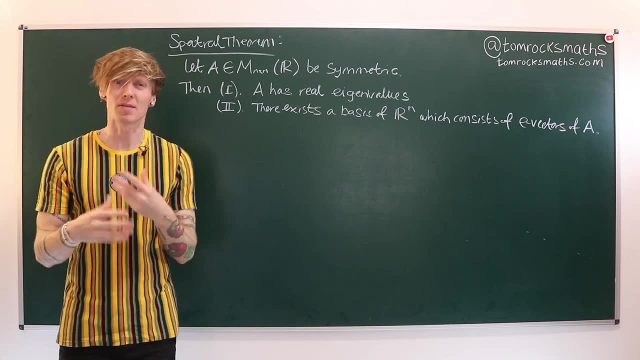 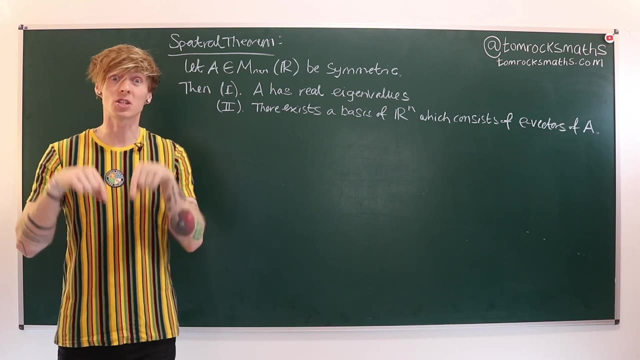 they can be quite complicated and once you're working with diagonal matrices, things are a lot easier To really see the power of the spectral theorem in action. I recommend checking out the exercise videos from ProPrep, which are linked in the video description below this box. ProPrep is: 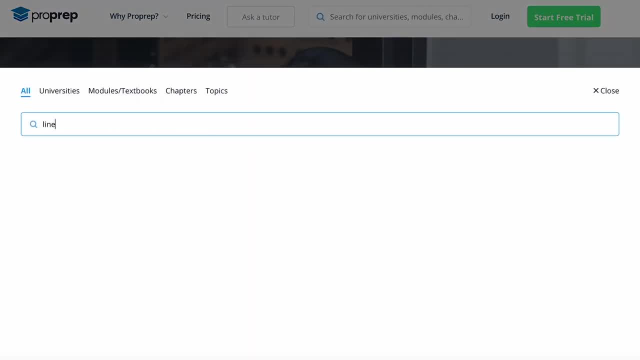 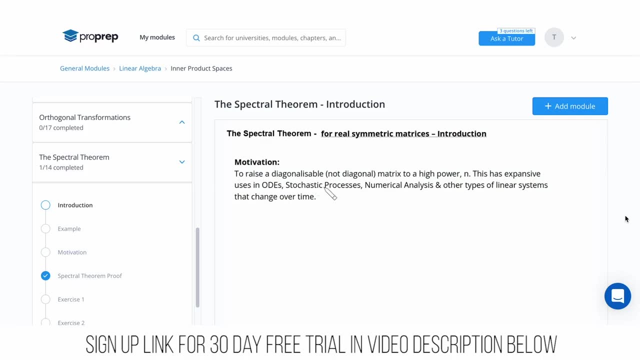 an online resource that provides you with a lot of information about the spectral theorem in action. ProPrep provides customized tutorials for students looking to improve their skills in stem-based subjects. There are 10 exercises on the spectral theorem, which each have a solution video. 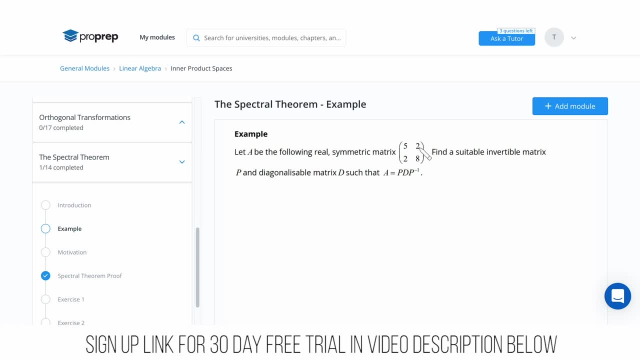 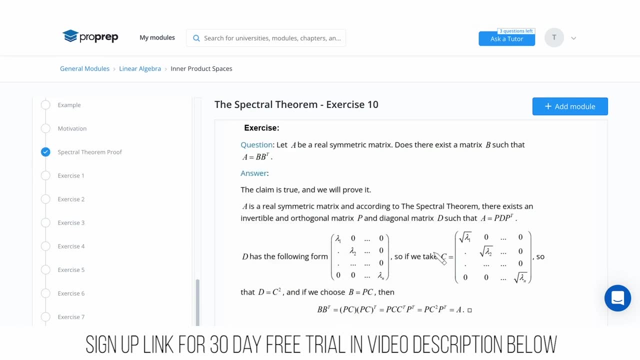 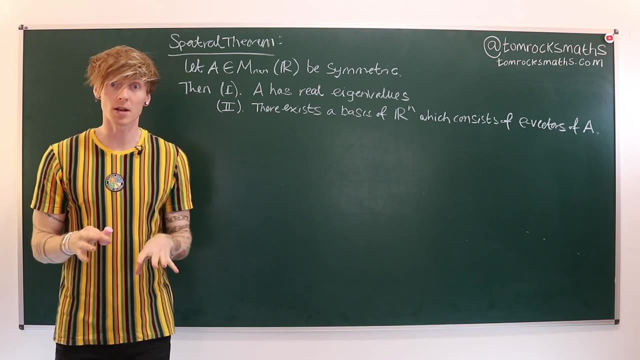 giving you a step-by-step breakdown of how to answer the question. Simply click the link in the video description to sign up for a 30-day free trial to see just how much ProPrep can help to streamline your learning. Okay, time for the proof. We are going to start with. 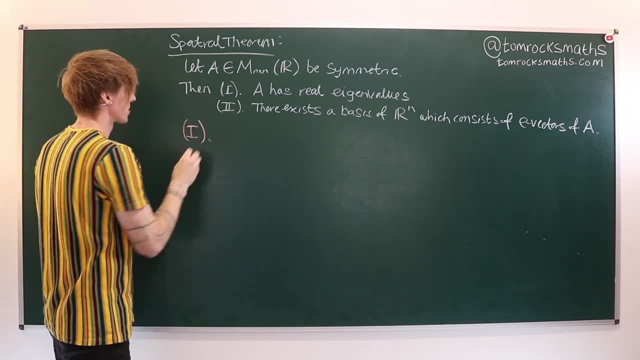 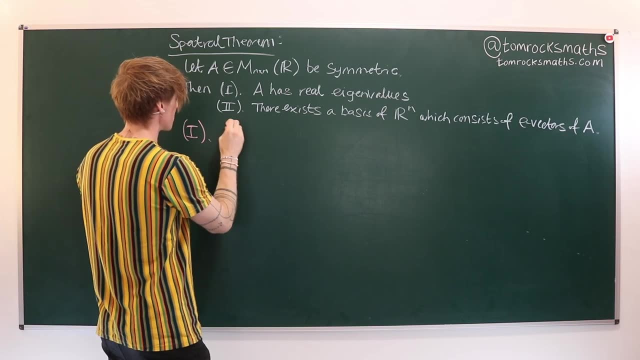 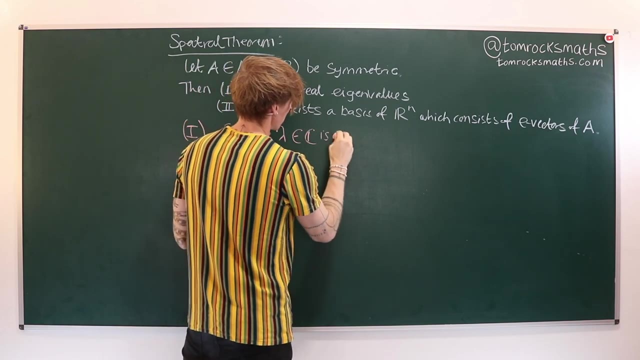 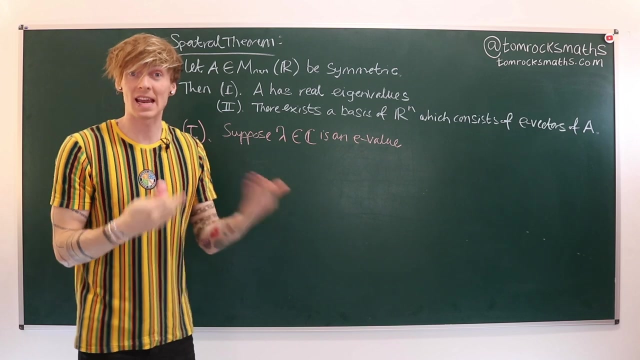 part one showing that the eigenvalues of a symmetric matrix are real. And the way we do this is we start by supposing lambda. suppose lambda belonging to C is an eigenvalue. So you'll notice that we are not making any assumption that lambda is real at this stage. 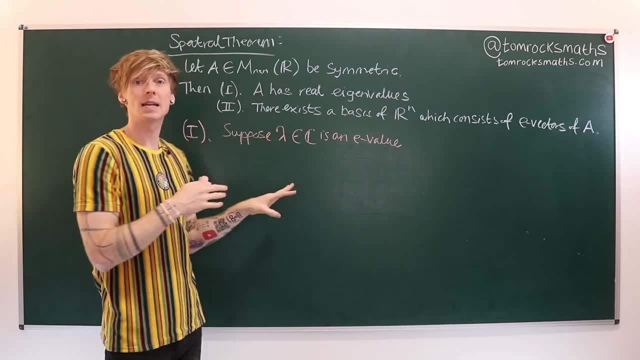 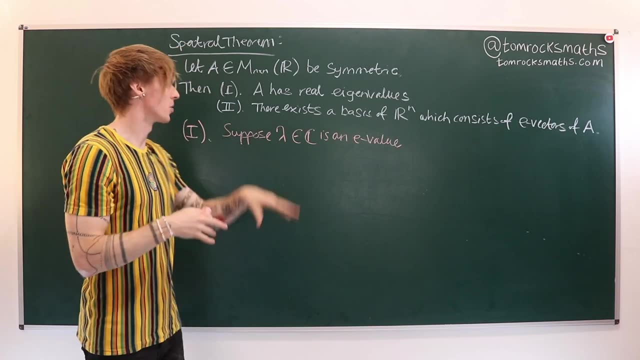 that's what we're trying to prove. But since we know that lambda is a root of the characteristic equation, we therefore, by the fundamental theorem of algebra, know that it must belong to C, the complex numbers. So we're going to show that, in fact. 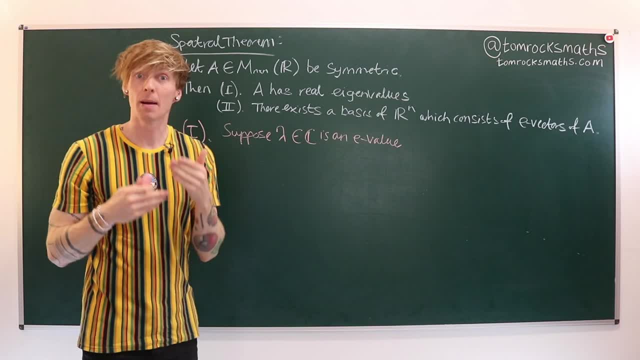 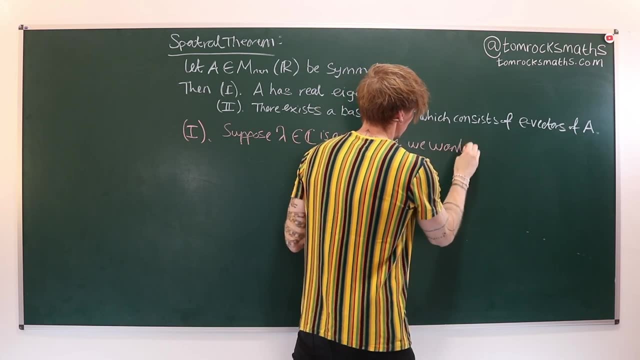 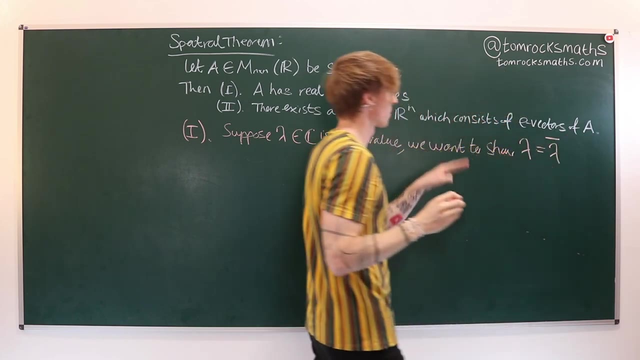 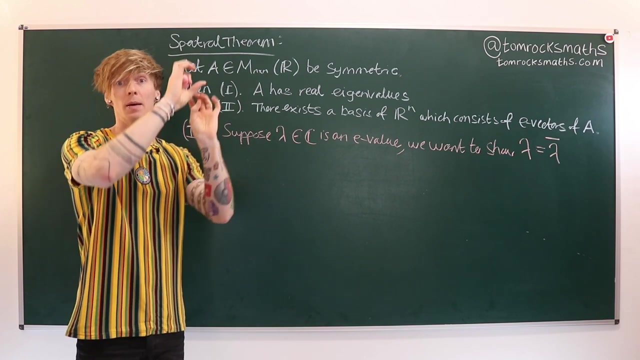 it has to be real. We can rule out anything with an imaginary part. And the way we do that is we want to show. we want to show that lambda is equal to lambda bar, where lambda bar is the conjugate, Because to conjugate a complex number you change the plus or minus i component. 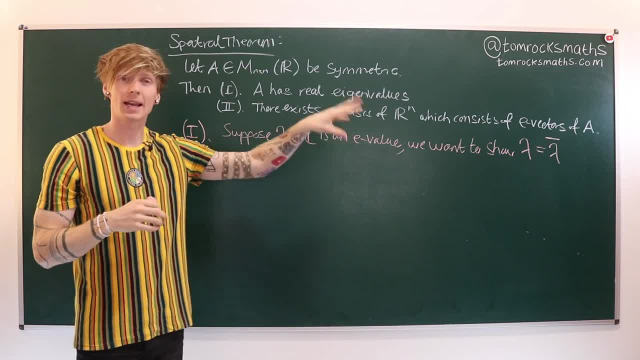 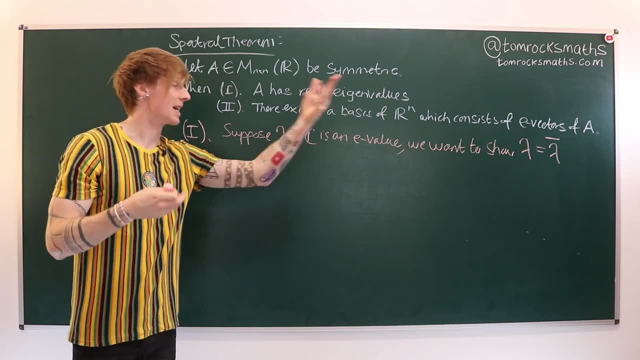 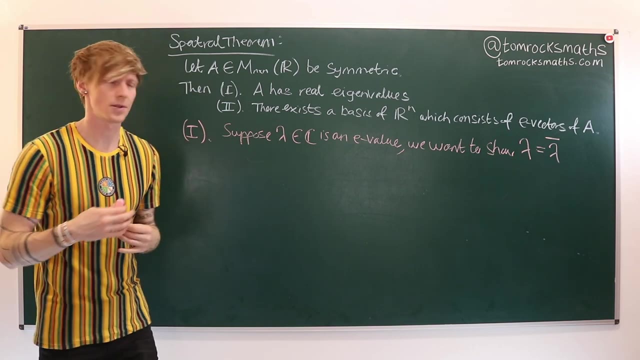 you swap its sign. So if we show that lambda and lambda bar are equal, that must mean the imaginary part is in fact zero and therefore it isn't changed. when you take that conjugate, Our starting point is going to be the eigenvalue equation. So this tells us that a times your eigenvector. 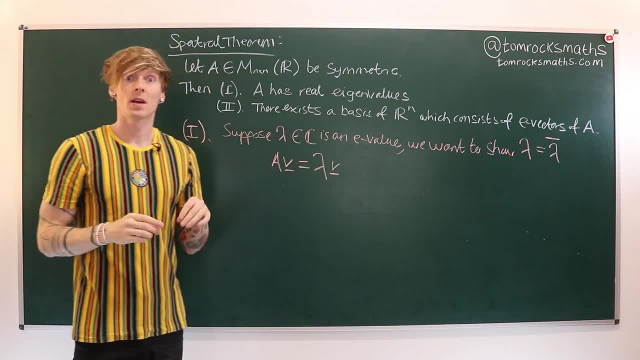 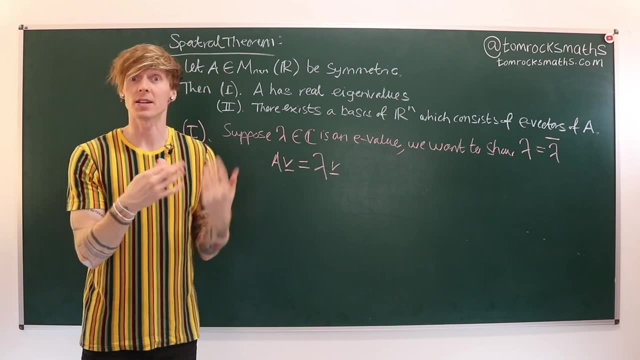 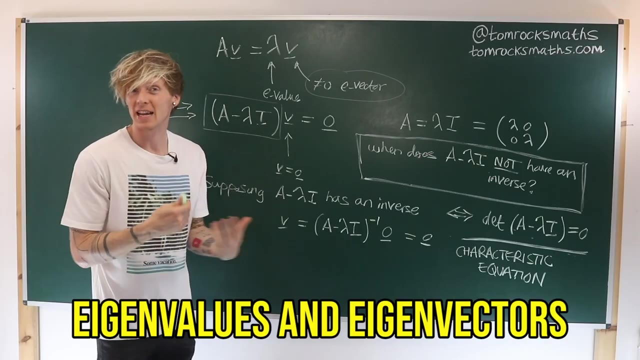 is lambda times v. Now, if you're not sure where this has come from, or you're not sure of the terms eigenvalue, eigenvector, characteristic equation or characteristic polynomial, then I do cover all of these topics in the previous video in the Oxford Linear Algebra. 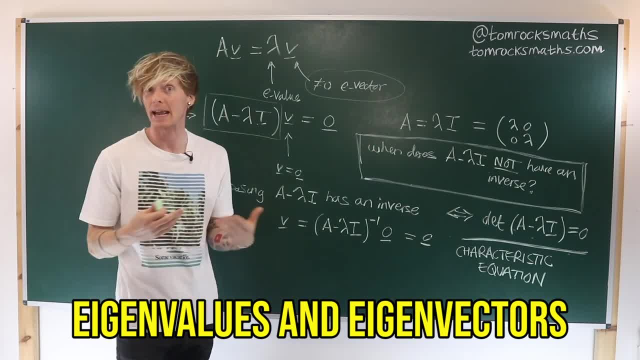 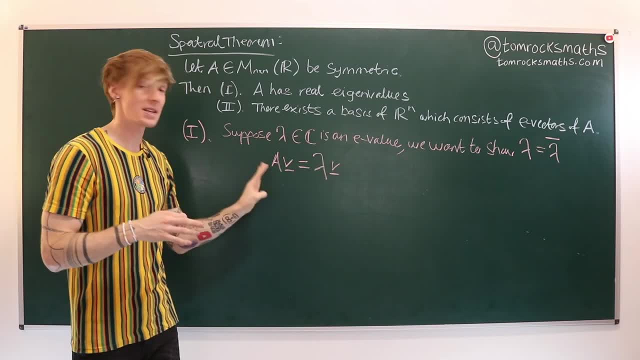 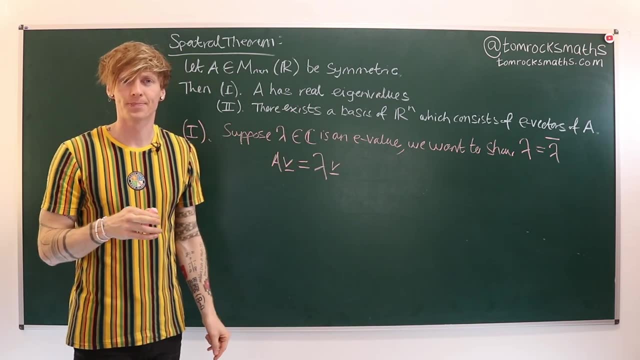 series which is called Eigenvalues and Eigenvectors. so I do recommend watching that, Otherwise I'm going to continue from here and in fact, it's going to be this equation which is going to allow us to deduce that lambda is equal to lambda bar. What we want to consider. 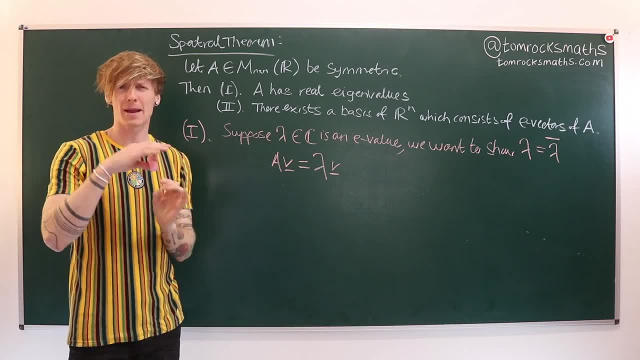 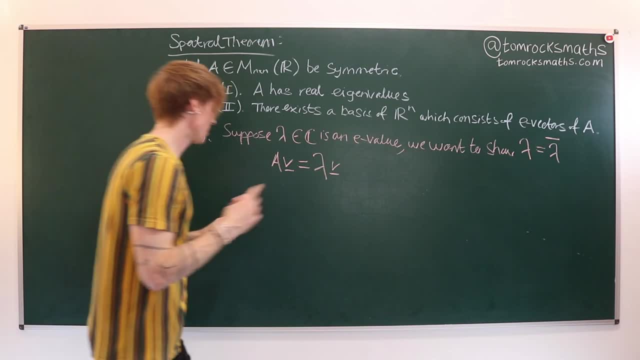 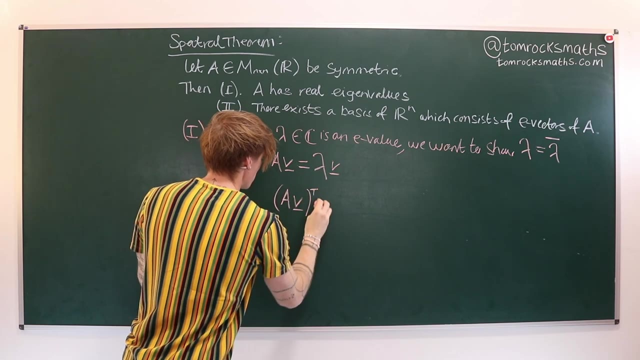 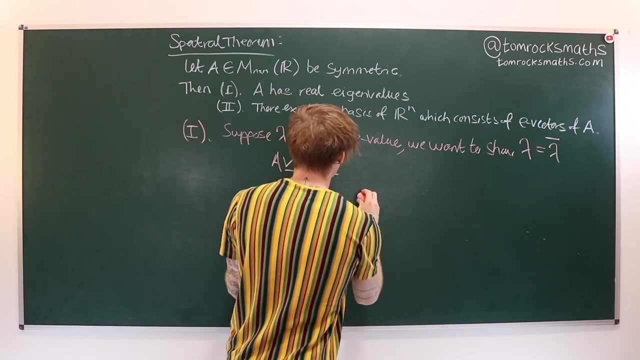 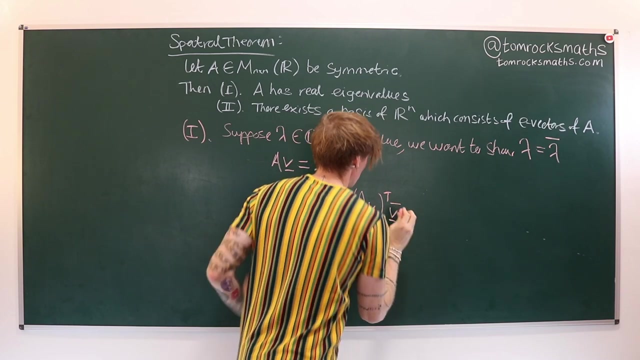 is the transpose of this equation and then post multiply by v bar the conjugate of the eigenvector v. So writing that out, we can say a v transpose and multiplied by v bar. From this equation that has to be equal to lambda v transpose multiplied by v bar. Now, taking the transpose, 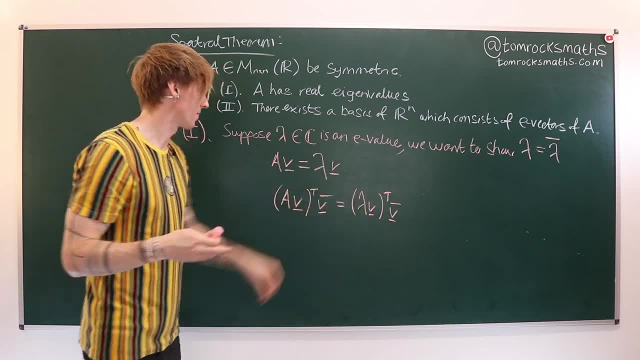 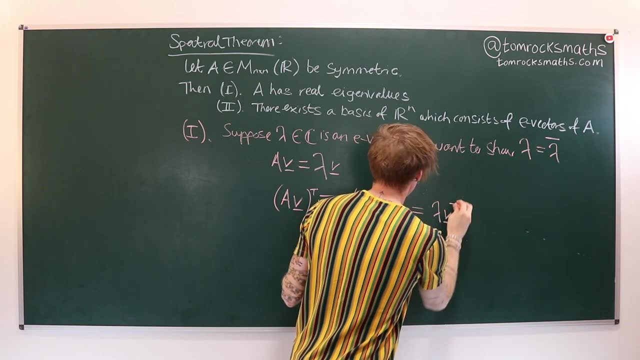 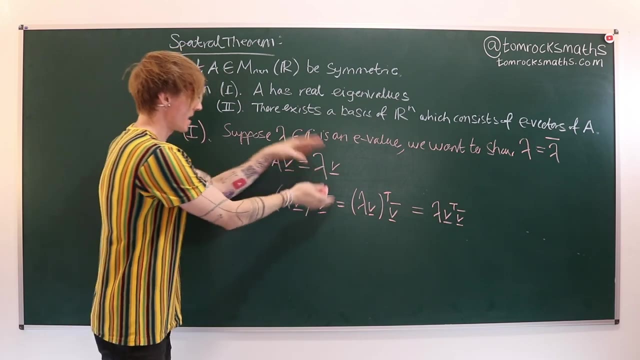 of lambda. that's just a number, so it's unchanged. and then v becomes v transpose, So that's actually equal to lambda times v- transpose, times v bar. And that's going to be our first way of evaluating this particular expression, So I'm going to label that with a one. 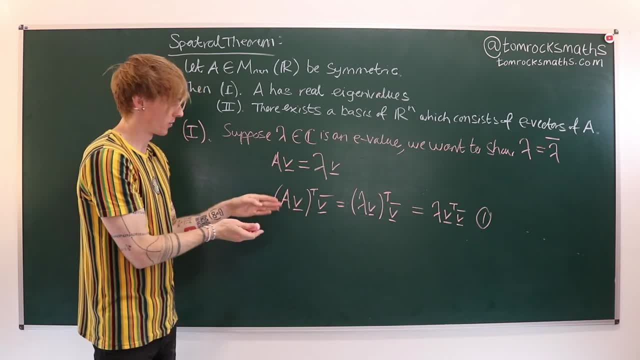 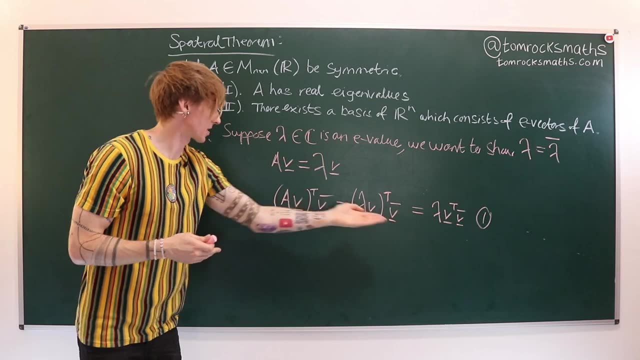 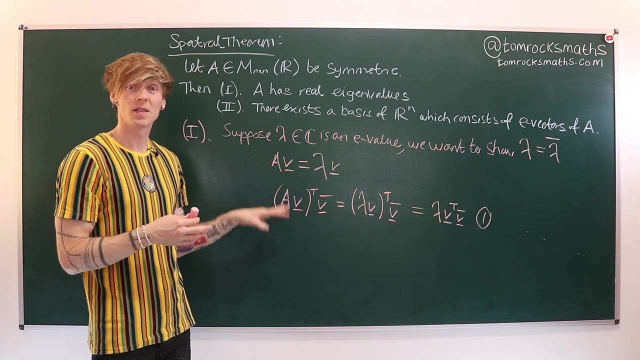 Now, what we've used here was actually to substitute for a v equals lambda v inside the bracket, and then expand that out and get our first expression for a v: transpose: times v bar. Now, alternatively, I can also expand this transpose, So I have two components multiplied. 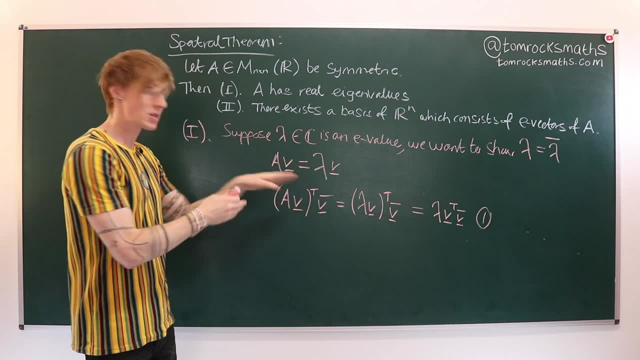 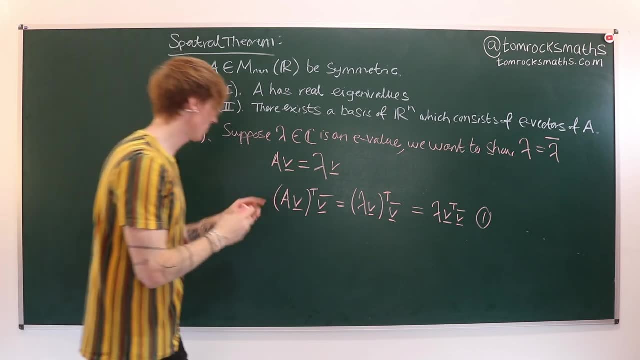 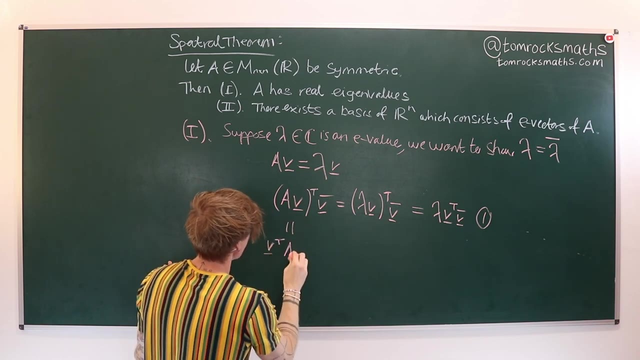 together and then transposed Outside the bracket. So the way you deal with that is you actually swap their orders and put a transpose on each of them individually. So if I do that, this is also equal to it's going to be a v transpose, a transpose, and then I still have my v bar. 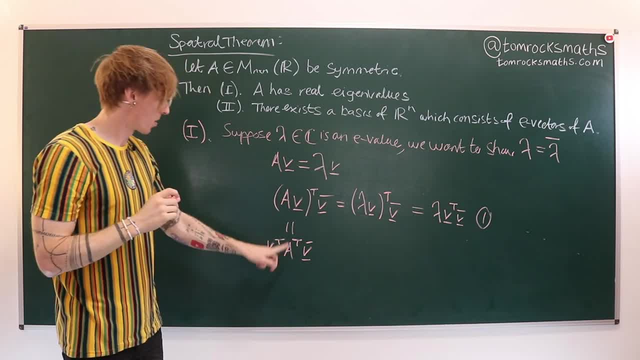 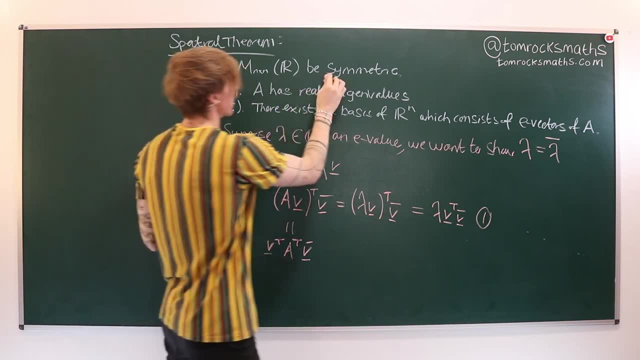 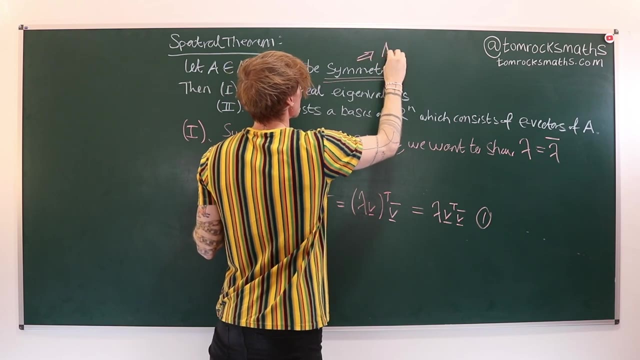 at the right hand side. Now, a is a symmetric matrix. We have yet to use that, and that's clearly going to be an important part of the theorem. So if a is symmetric, what that means is that a is equal to its transpose. So all the entries above the 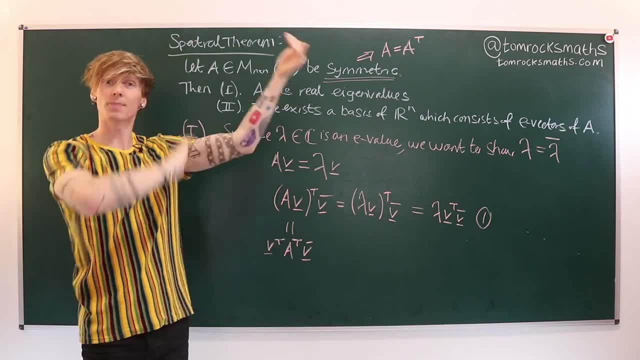 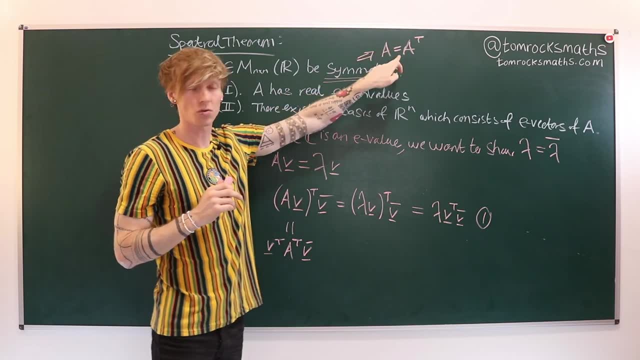 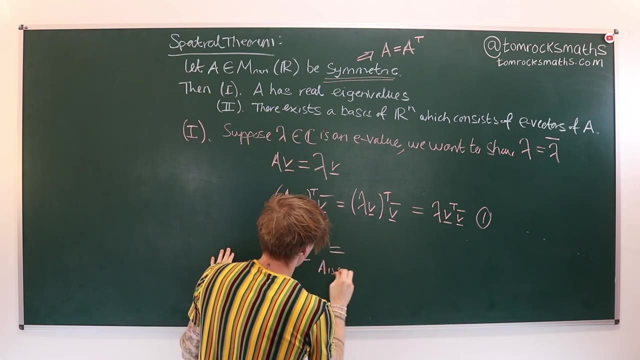 leading diagonal are the same as they are below. So when you transpose it it's like reflecting in that leading diagonal. So since this is true, I can replace a and say: well, a is symmetric, We can actually replace that. So we actually get now v transpose, times a times v bar. 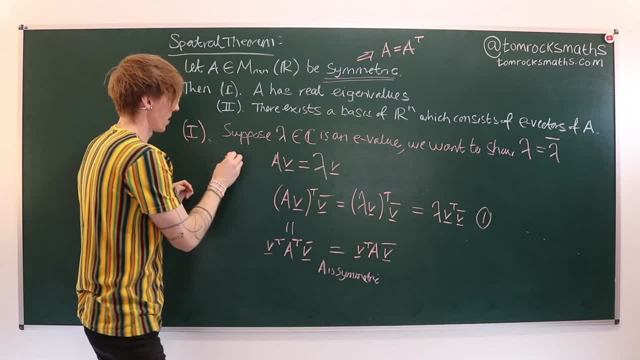 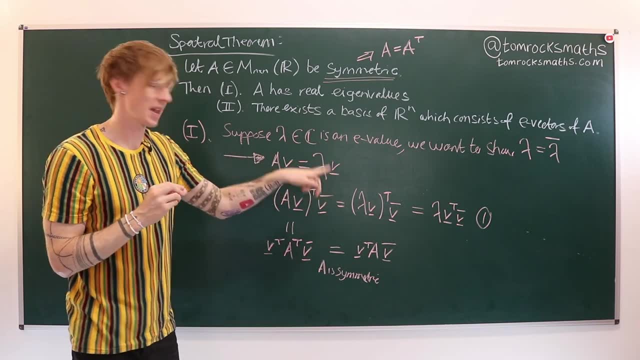 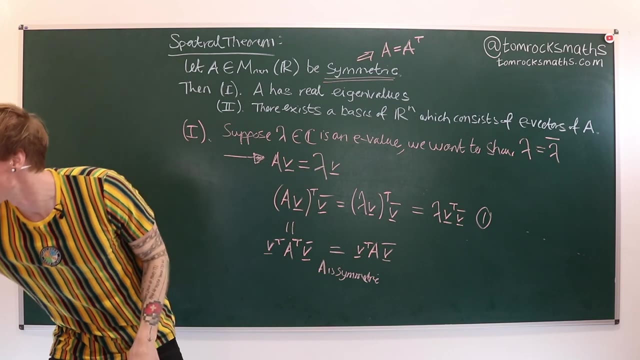 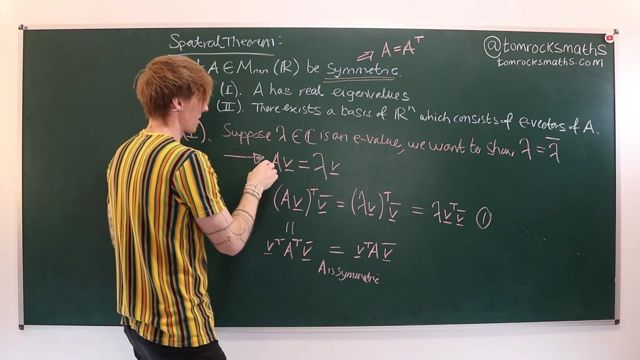 But then we also know from our eigenvalue equation here that we can conjugate this and get a result involving a and v bar. Because if I conjugate this equation- and I'm going to do this in a different colour just to emphasise that it's another version of this result- So if I conjugate this, a is real, a has real entries. 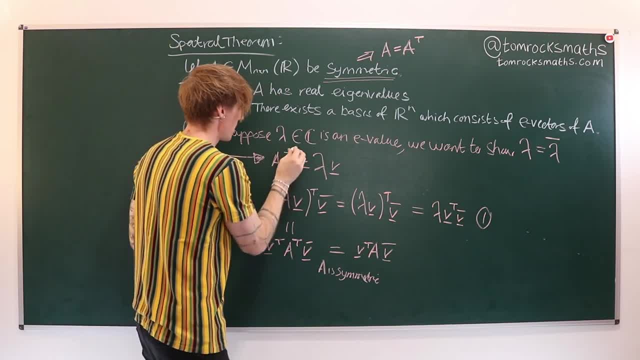 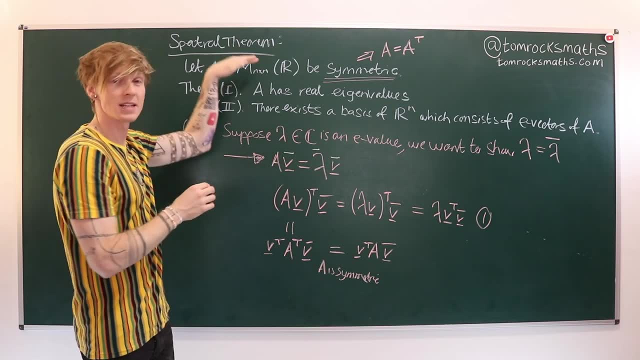 So conjugating a does nothing. So I've got a bar here, a bar here and a bar here. So this is the conjugate version in this particular instance of a being real. So now I can substitute for a, v and v. 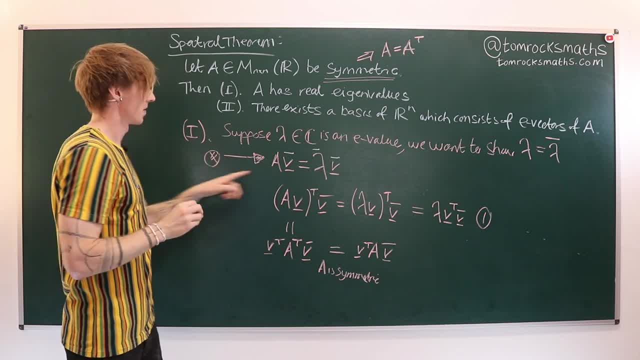 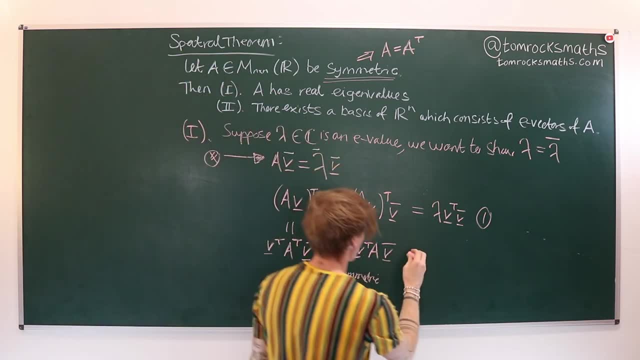 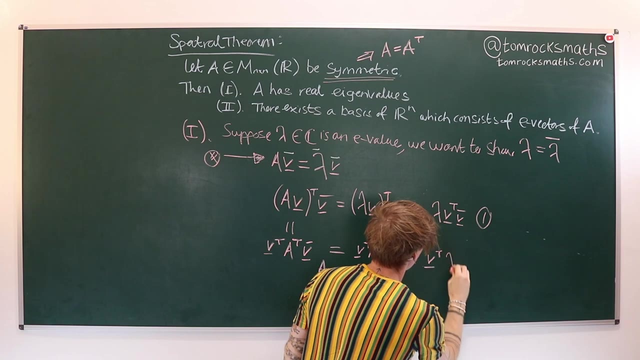 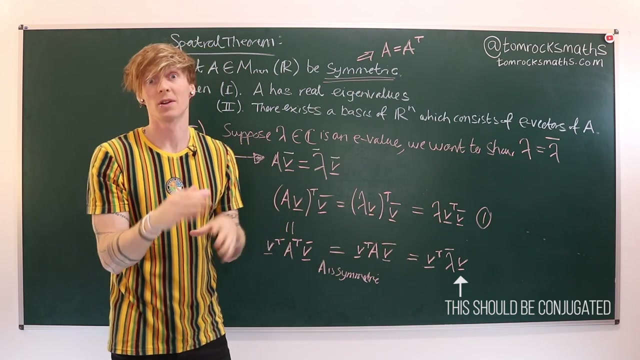 v bar from what I'm going to call star This equation here, the conjugated version of the eigenvalue equation. So substituting down here this is now v transpose a times v. bar is lambda bar v bar, lambda bar v bar. But now lambda bar is just a real number. Well, we don't know, it's. 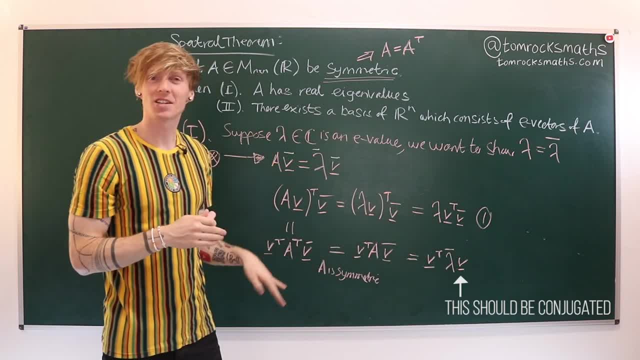 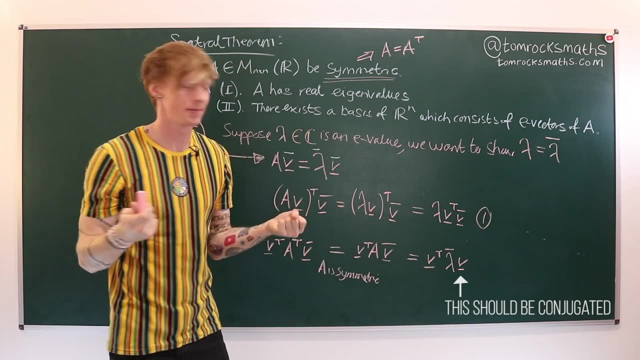 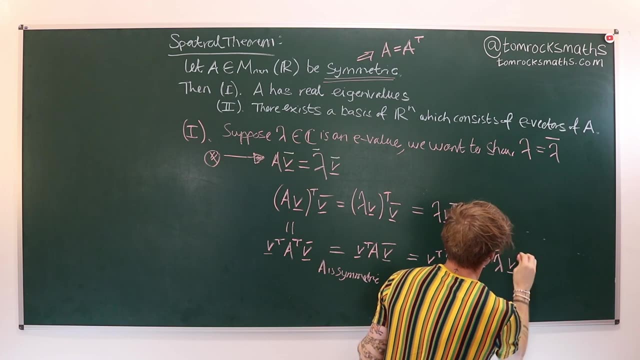 real, yet It's a number, It's a constant, So I can actually bring that to the front. You have a constant multiplying a vector or a series of vectors. You can always pull out that constant. So this is actually just equal to lambda bar, times v. transpose times v- bar And that's going. 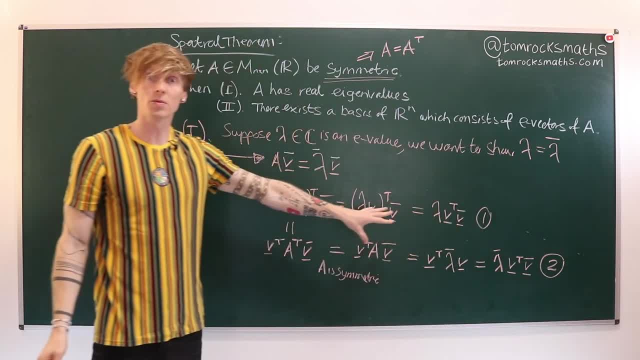 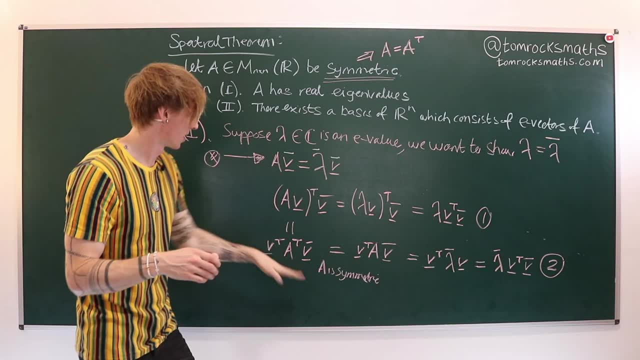 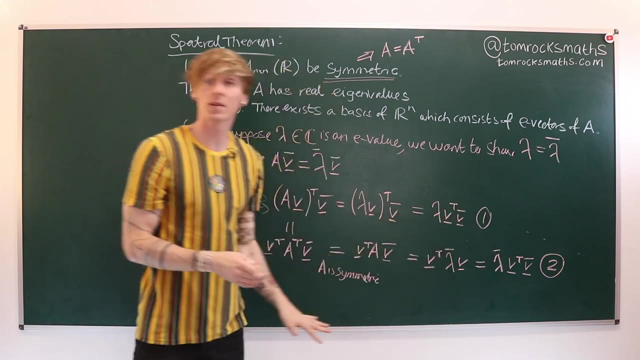 to be equation two. So one and two. both expressions over here are actually equal to one another Because we can follow the equal signs from our original starting expression, which is this: one of a, v, all transpose times v, bar. We've got two equivalent ways of writing that expression. 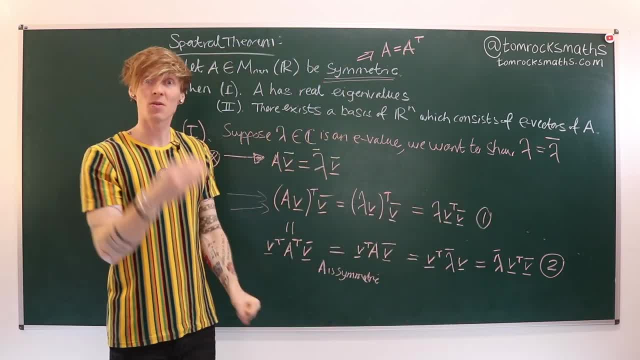 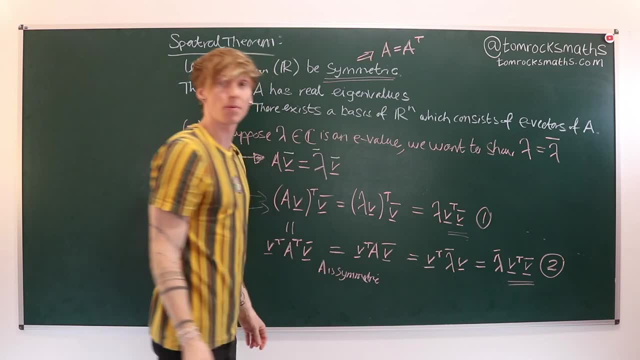 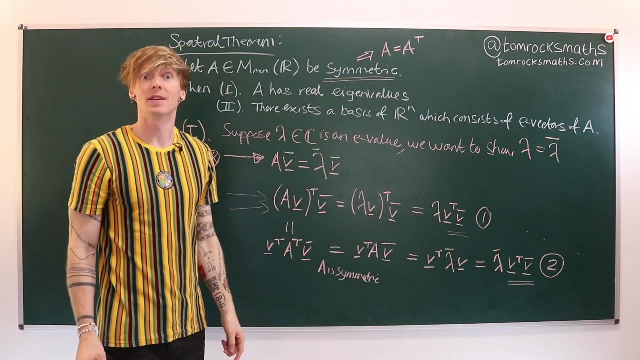 So these are equal. Now we're almost there because they both have the same post-multiplication product. They're both lambda times v transpose v bar and it's lambda bar times v transpose v bar. So we can cancel that product of the v's. 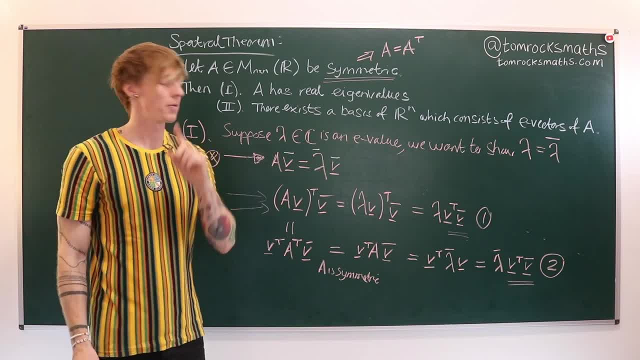 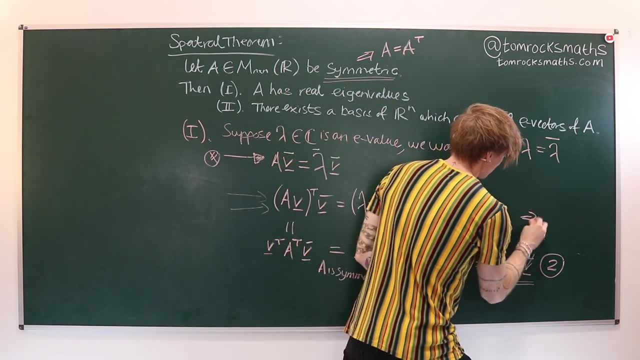 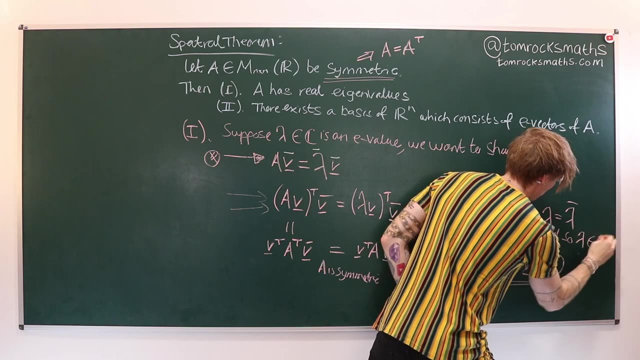 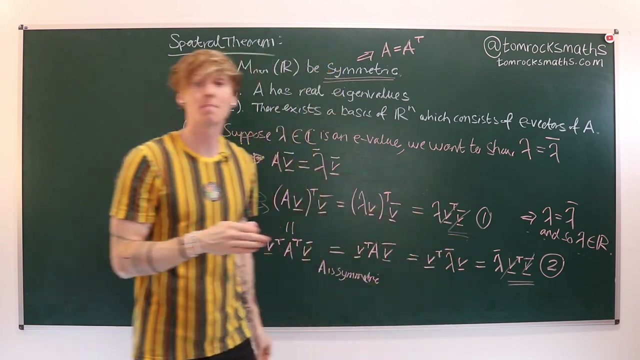 provided it's non-zero. Now, fortunately, it is non-zero. So that's what we do: We cancel these, and that tells us that lambda is equal to lambda bar, And so lambda belongs to the reals, which is what we wanted to show. But remember that does require v transpose times, v bar being. 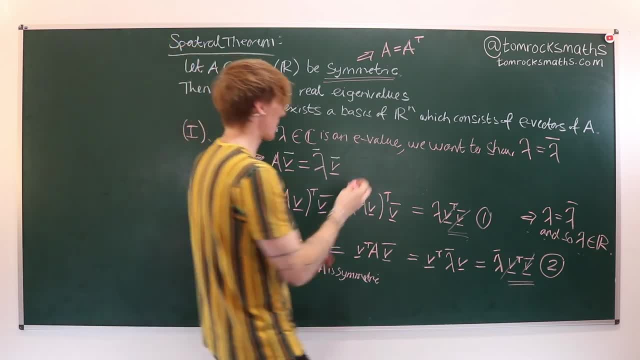 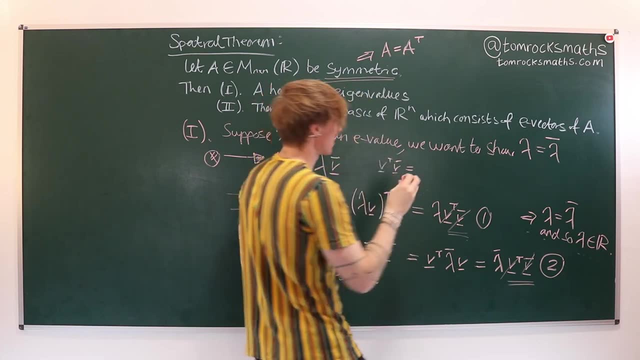 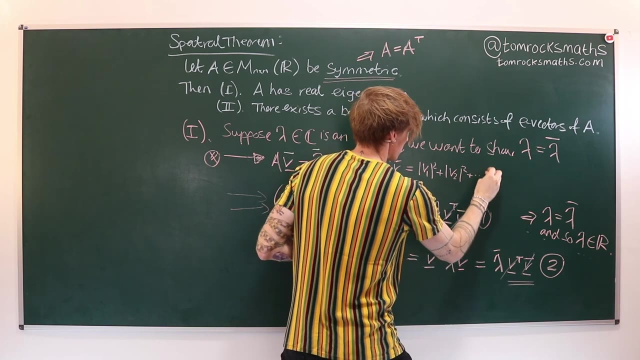 non-zero. It has to be true because when we calculate that if you did v transpose times v bar, that would actually give you the first entry modulus squared plus the second entry modulus squared plus dot, dot, dot up to the nth entry. 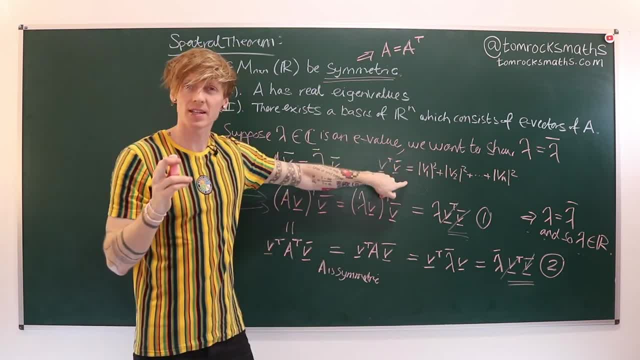 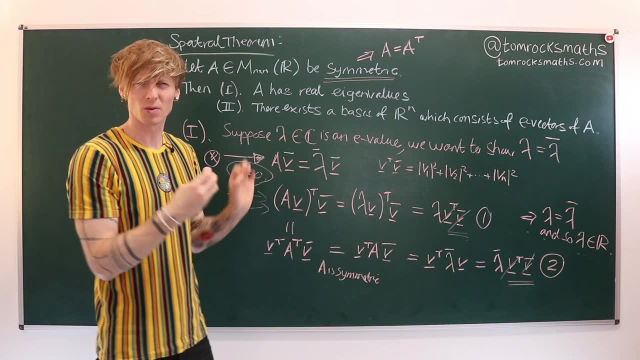 But we know that v is an eigenvector. so because it's an eigenvector, we actually know here that v is non-zero because it's an eigenvector. That's one of the rules of being an eigenvector. 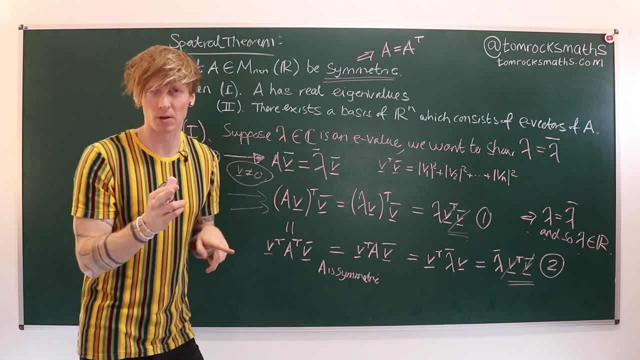 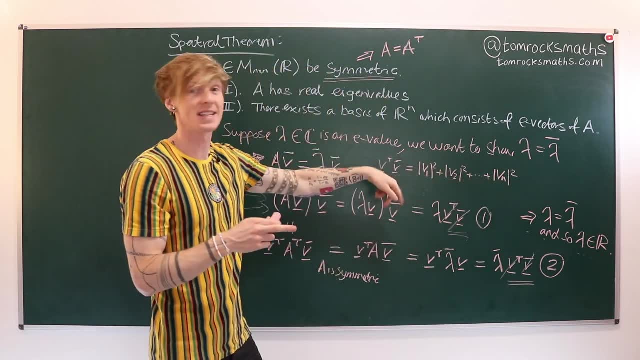 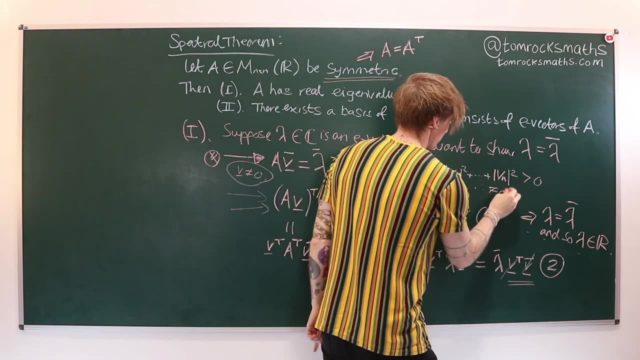 So because it's nonzero, that means it's not possible for all entries to be zero, and the only way this would be zero this product is if every single entry was zero. So this is strictly positive, therefore nonzero, and so cancelling over here was fine, and that's where we end up with the result. lambda equals lambda bar. 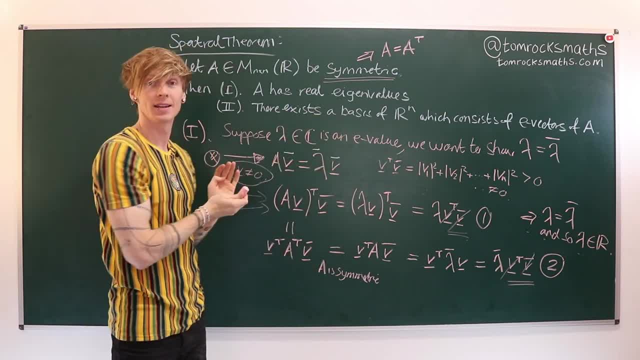 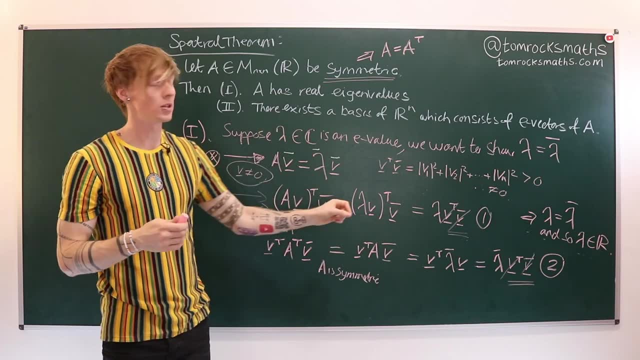 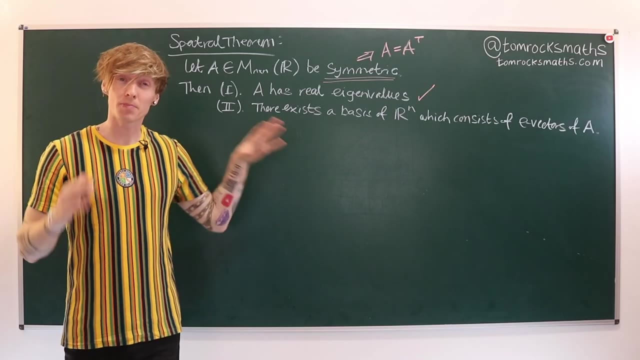 which shows that this generic eigenvalue, which we assumed originally could be complex, it turns out we've been able to show is in fact real, which completes the first part of our proof of the spectral theorem. For the second part of the proof we're going to actually prove an equivalent result about the existence of. 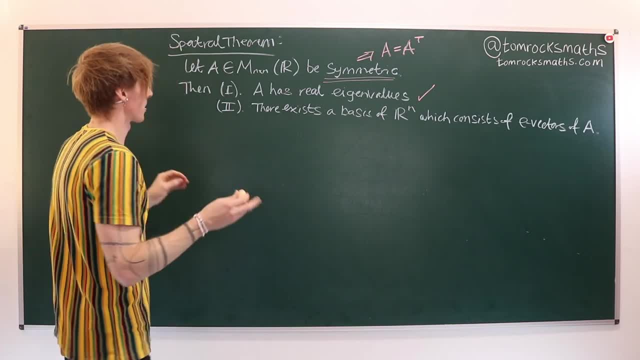 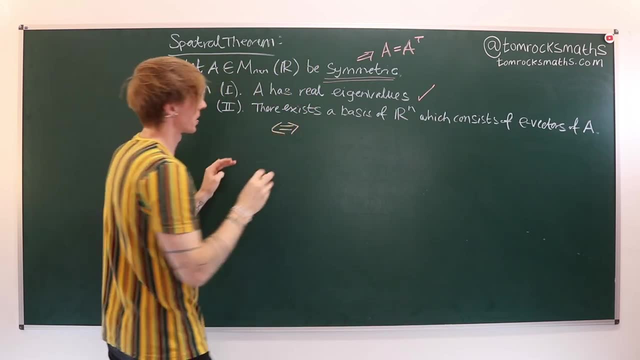 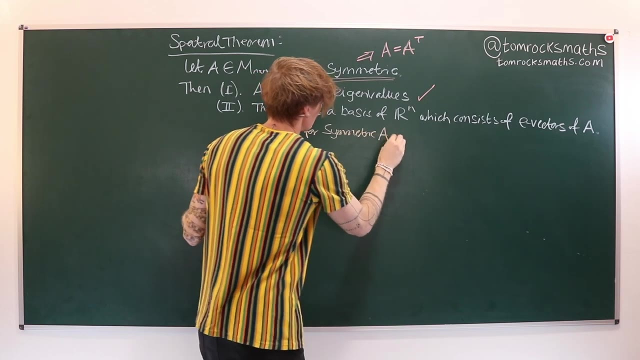 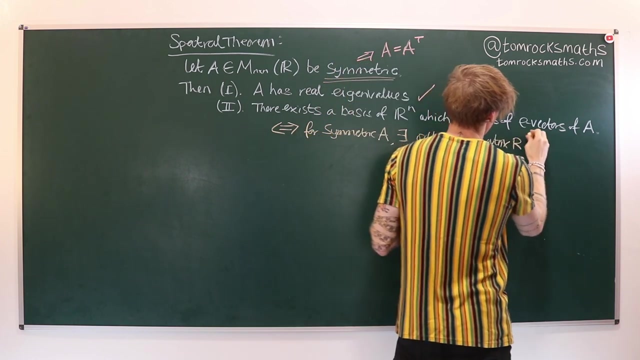 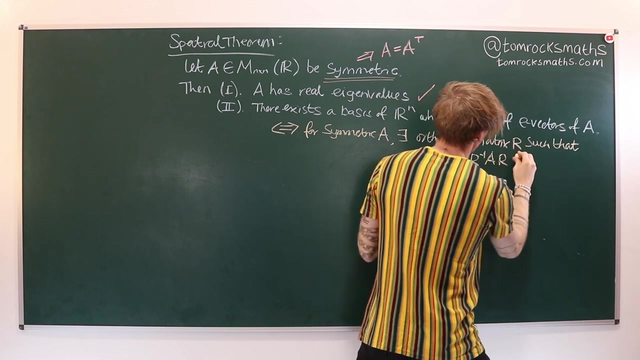 a basis of eigenvectors and that says the following: There exists a basis of Rm which consists of eigenvectors of A. That is in fact equivalent to showing that for Rm- symmetric A- there exists an orthogonal matrix, R, such that R inverse A, R is 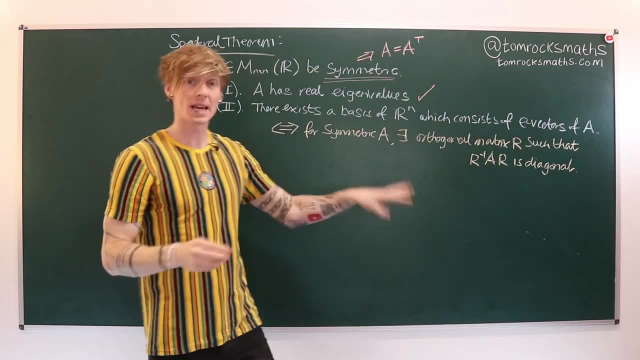 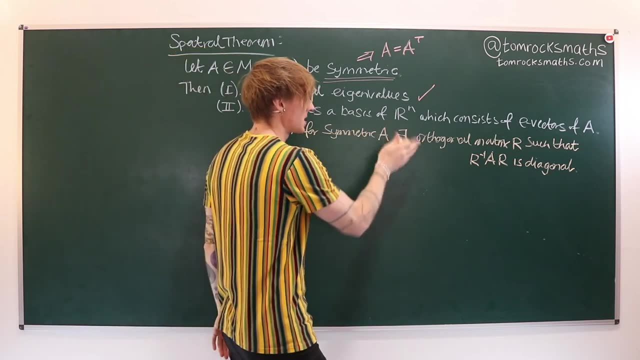 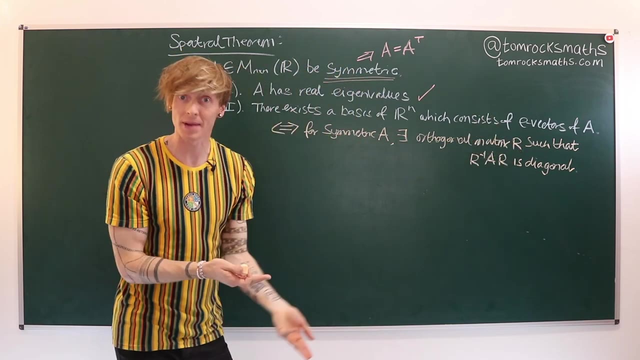 diagonal. So really, what we're saying here is there's going to be an orthonormal basis- we'll come to that in a moment- and in that basis we can actually change basis or we can create a similarity transformation between the matrices in order to make A become this diagonal matrix. So that is in fact. 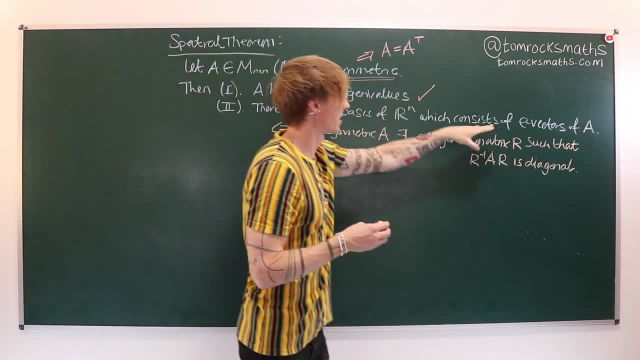 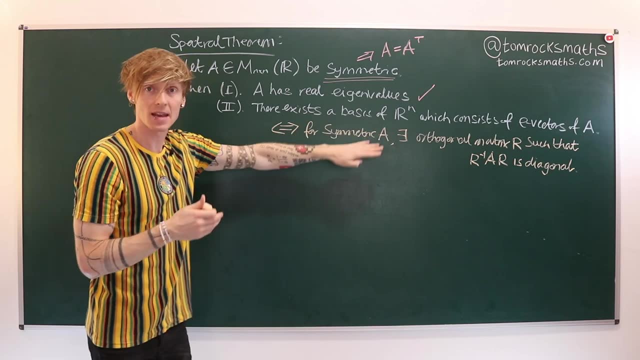 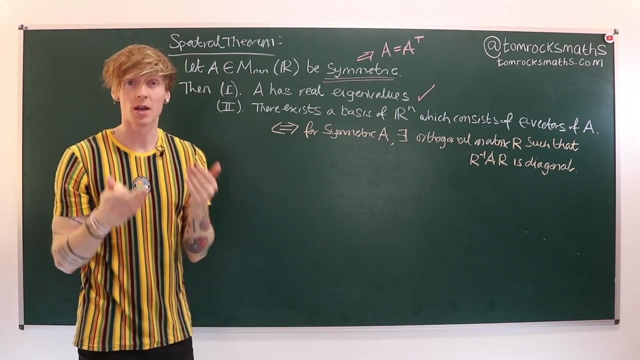 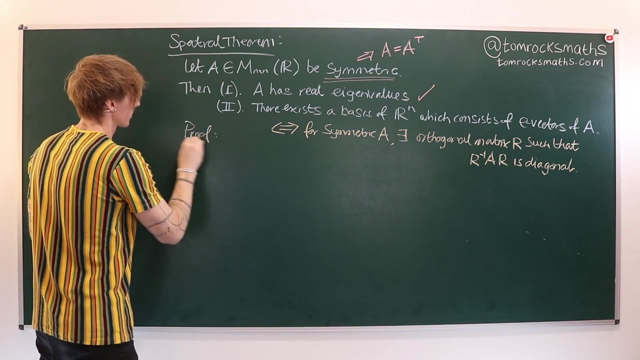 equivalent to showing that a basis of eigenvectors exists. So I'm going to prove the result in orange is true for symmetric A, and then that can be used as an equivalence to actually prove part 2 and therefore complete the proof of the full spectral theorem. We begin our proof as follows: Suppose lambda 1 is an. 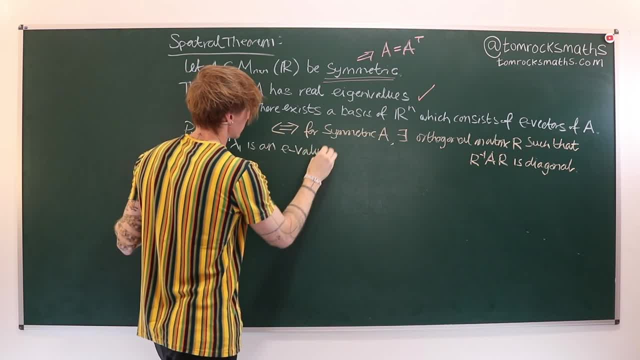 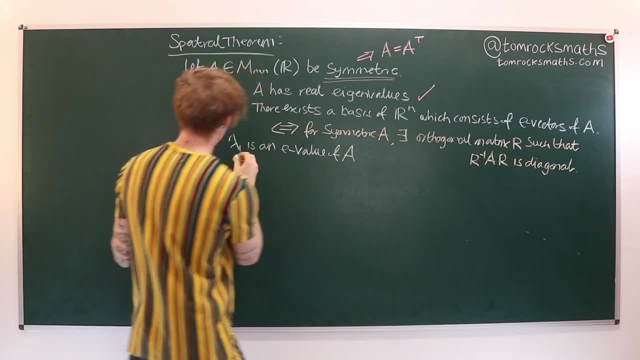 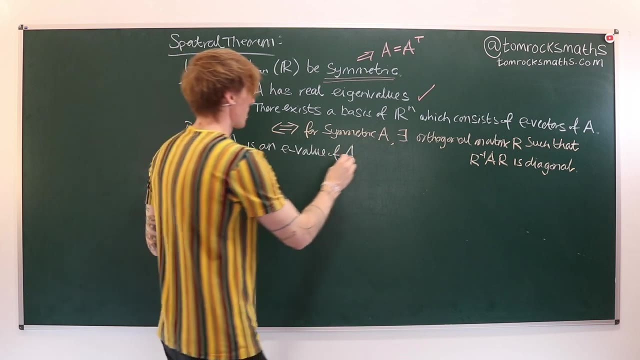 eigenvalue of the matrix A. So by part 1, which we've already shown to be true, we know that this is actually real. So let's just note that down At this stage. and it's going to have an eigenvector v1.. Now what we're going to. 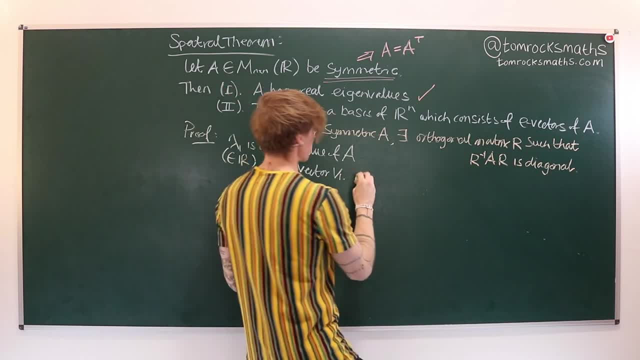 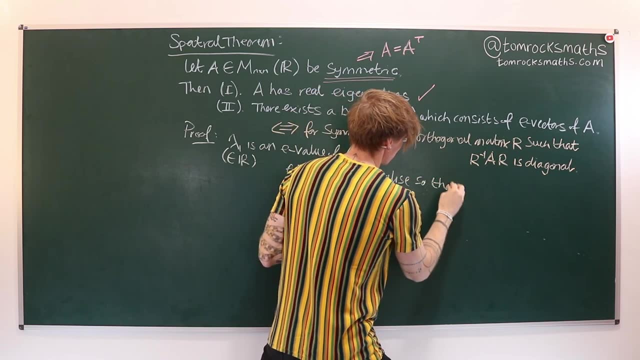 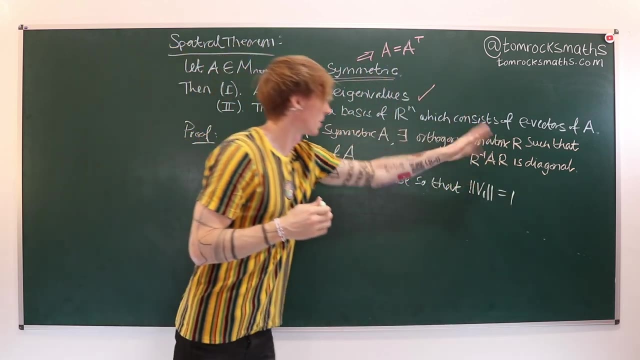 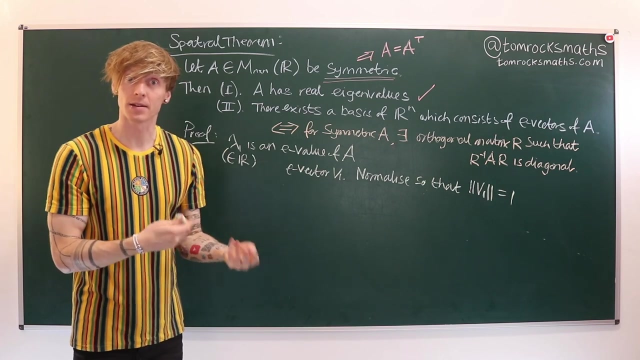 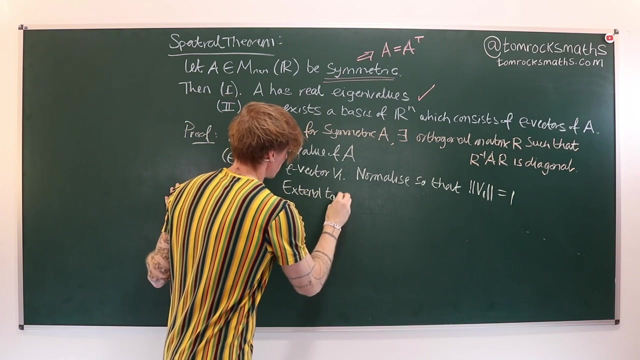 do with the eigenvector is we're going to normalize. So normalize this eigenvector so that the size of this- so the modulus v1, is equal to 1. So it is normalized, has length 1.. Now we're going to extend this basis. So extend to a basis, extend to a basis of Rn. 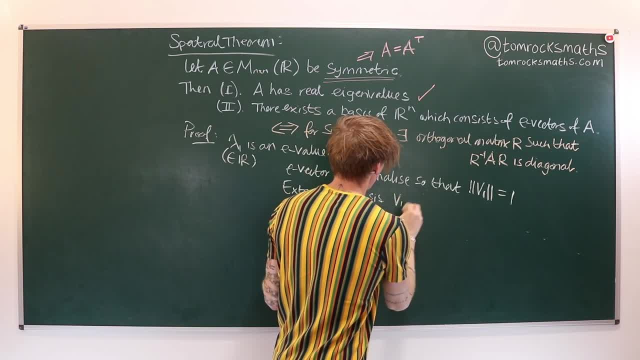 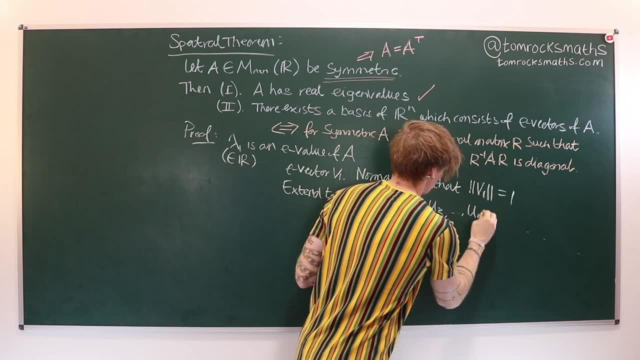 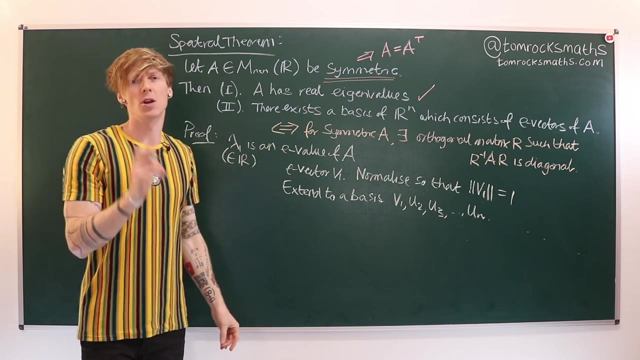 And let's call it v1,, u2,, u3,, dot, dot, dot, up to our nth vector, which we'll call Un. Now, I've purposefully labeled these others with uses because at the moment they are not normalized. They don't necessarily have length 1.. 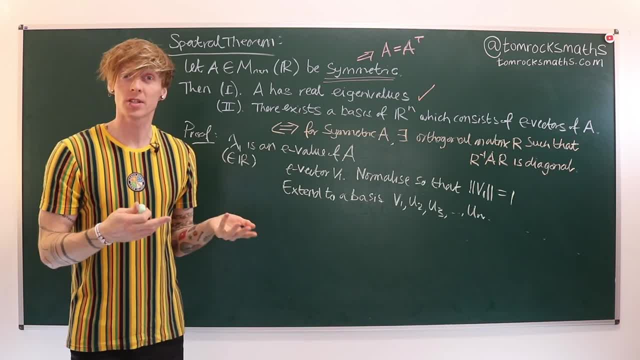 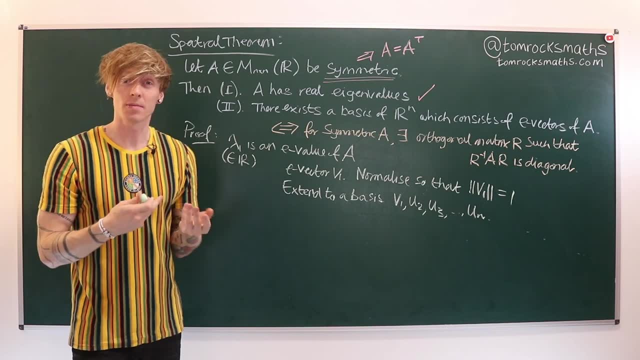 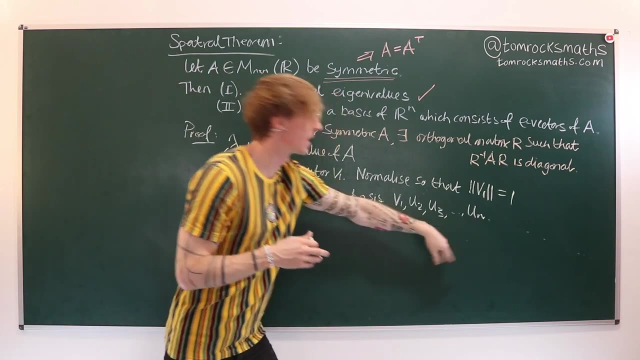 However, there is a very useful result called the Gram-Schmidt procedure or the Gram-Schmidt process, which actually gives an algorithm or a method, like a recipe, that you can follow, and it allows you to take a basis and turn it into an orthonormal basis for any 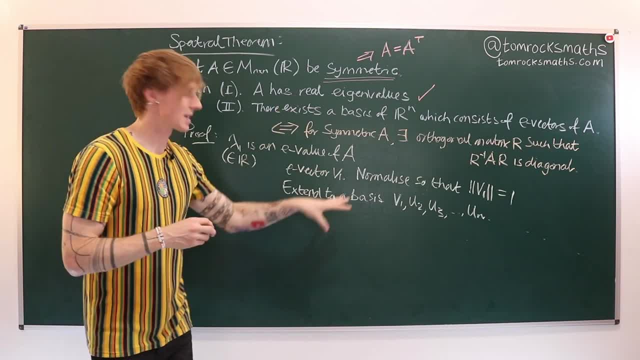 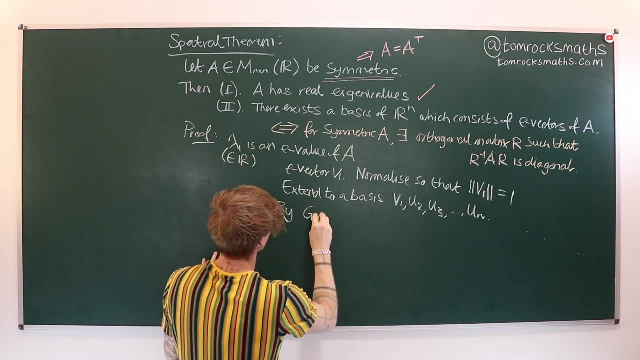 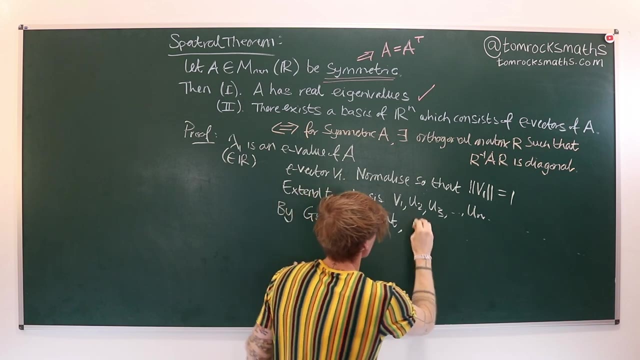 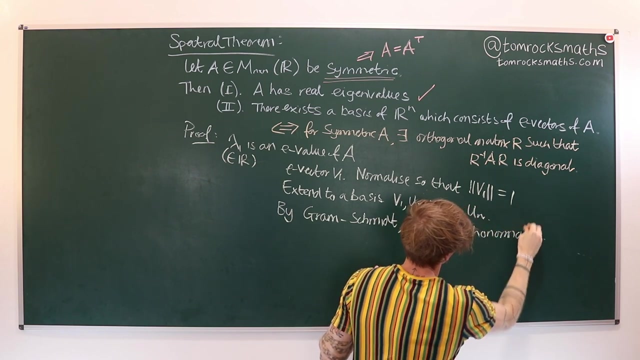 finite in a product space. So that is actually applicable here. So we can say: by Gram-Schmidt- and I will talk more about this in just a moment- we get an orthonormal basis. orthonormal basis and this is given by v1, v2, up to vn. 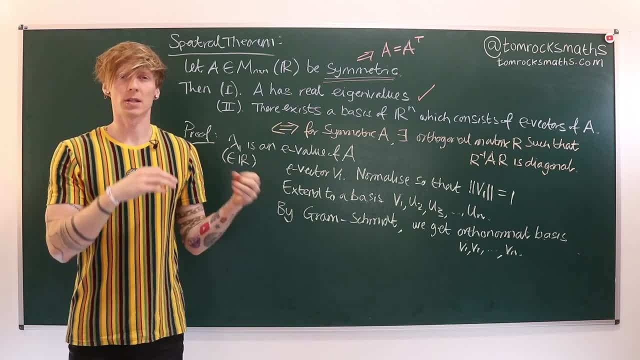 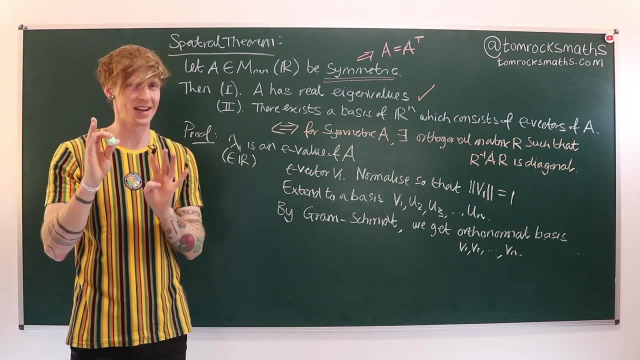 Now I'm not actually going to say any more about the Gram-Schmidt process in this video. I may feature it in a future video. we'll see no guarantees, But if you want to find out more about the Gram-Schmidt process, you can go to the link in the description below. 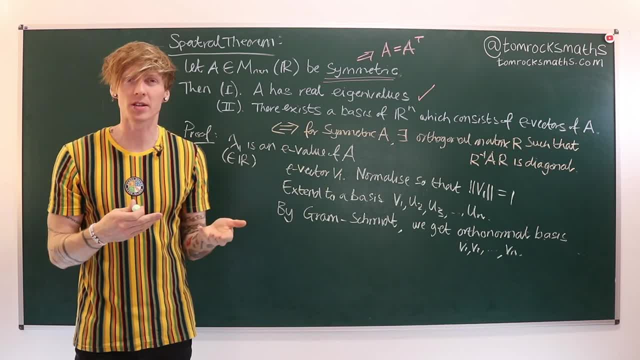 So if you want to find out more about the Gram-Schmidt process, you can go to the link in the description below. If you want to find out more about the Gram-Schmidt process and how that algorithm works, then there is a series of videos on ProPrep, all of which are again linked in the video description. 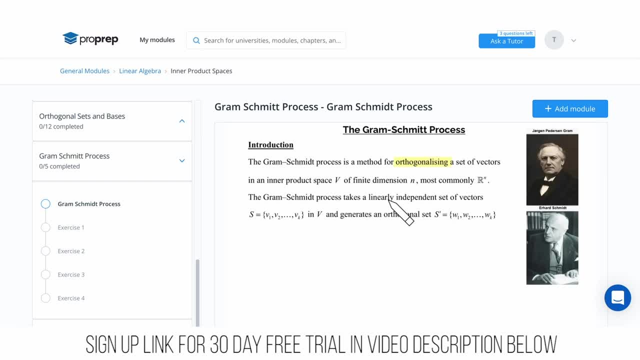 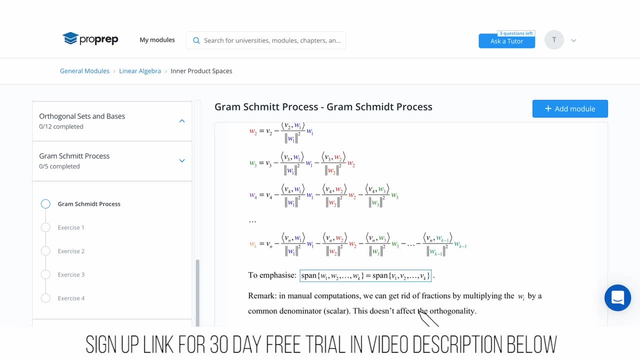 There's an explanatory video which shows how the procedure works, as well as four exercise videos which ask you to use it to actually formulate, with real numbers, an actual orthonormal basis. So if you would like to find out more about Gram-Schmidt, 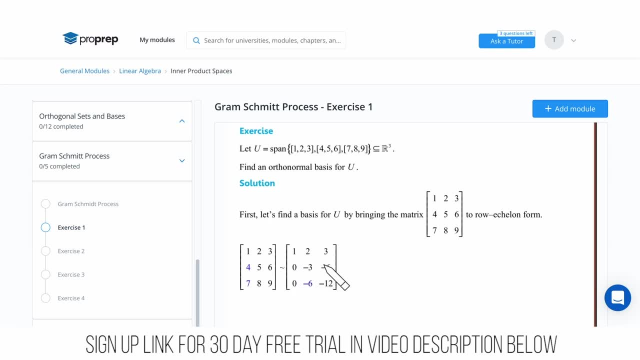 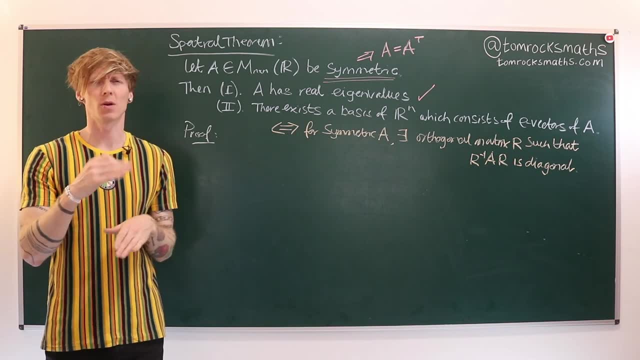 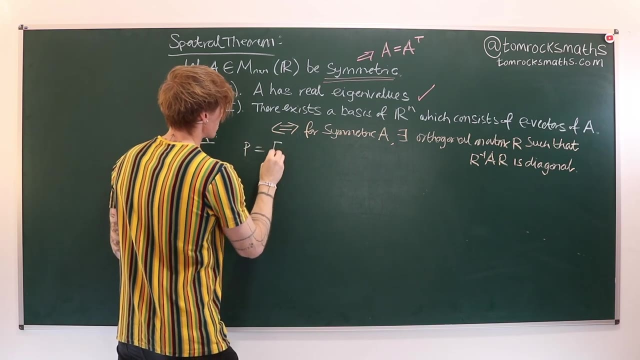 then make sure you check out the links in the video description And remember to sign up for your free 30-day trial. Now that we have our orthonormal basis, given by v1 up to vn, the next step is to formulate the matrix P, which is created by putting the basis vectors as the columns. 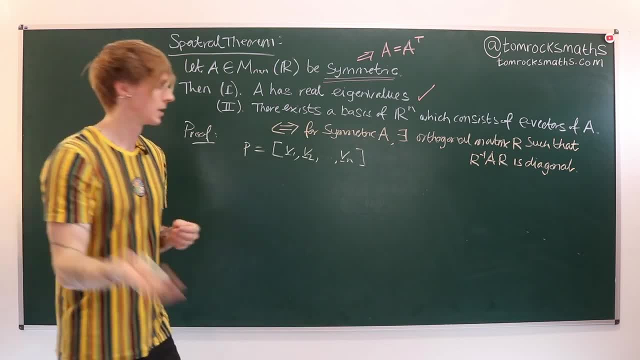 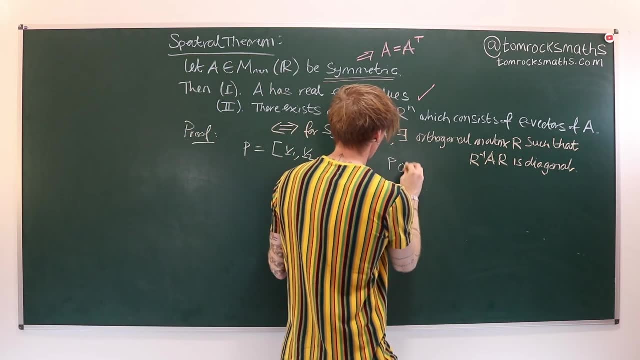 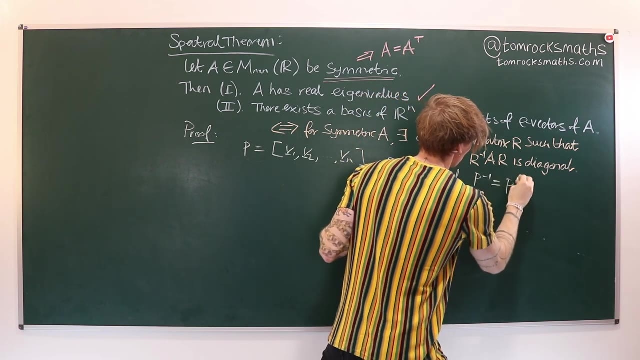 Now important properties of P to note are that P is orthogonal because these are orthonormal basis vectors. So P is orthogonal, which means that P inverse is equal to P transpose. That's what it means for a matrix to be orthogonal. 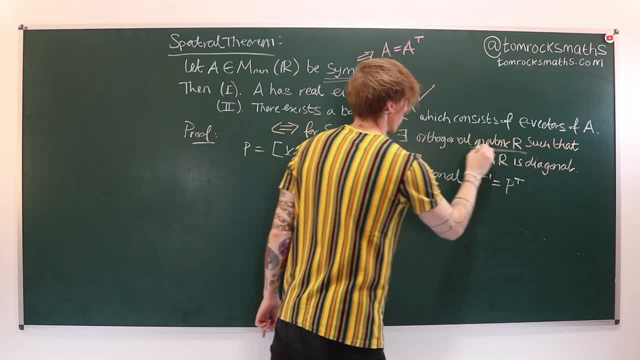 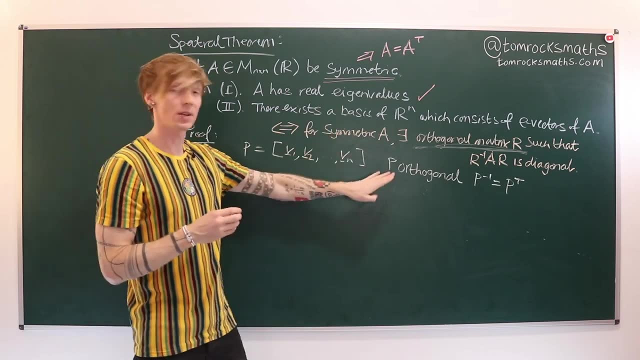 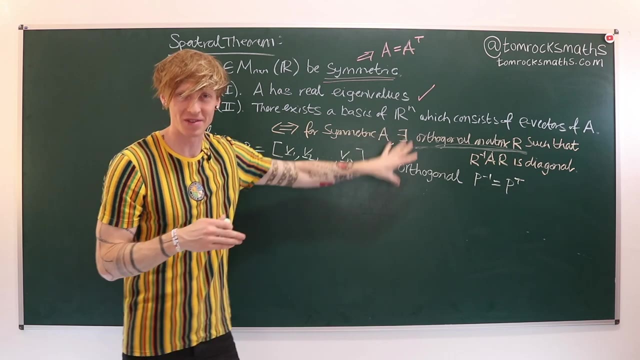 Now you will notice that we're trying to show up here that we have an orthogonal matrix R, such that the combination of it with A is diagonal. Now I am purposefully using P and not R because there are some further steps, So I will eventually relabel something involving P as R, but that is kind of the relationship. 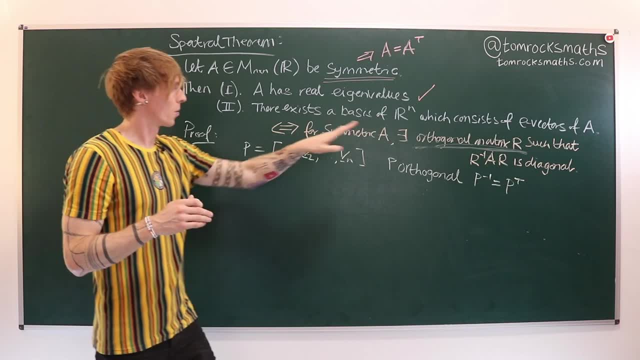 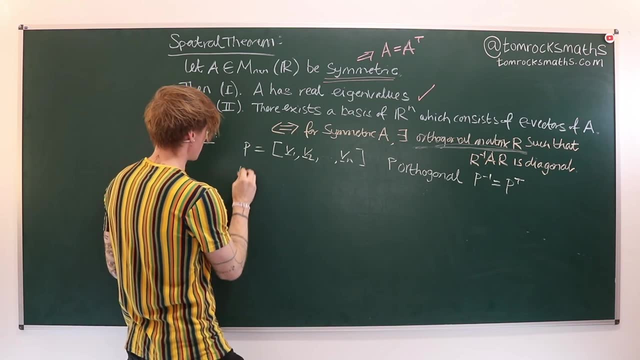 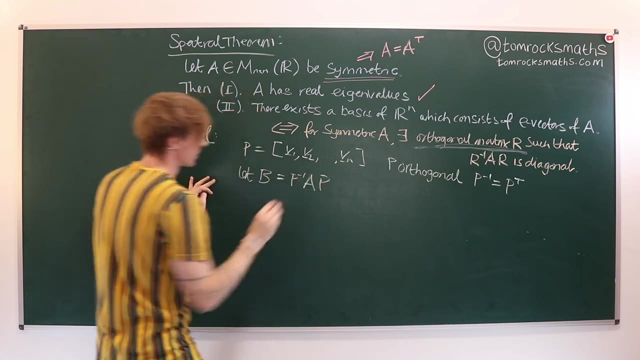 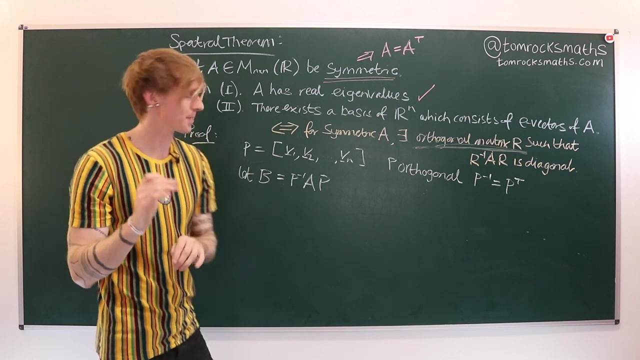 between these two Now. we therefore want to look at what is P inverse A R. so let's call that B. So let B be equal to P inverse A P. So again, this is sort of playing the role of R, but it's not quite the Finnish version. We will get to that. So we want to show that this is. 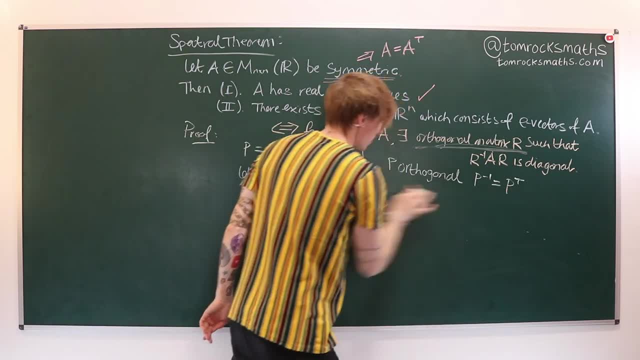 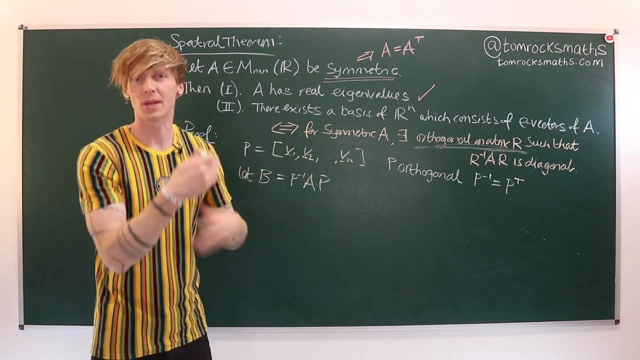 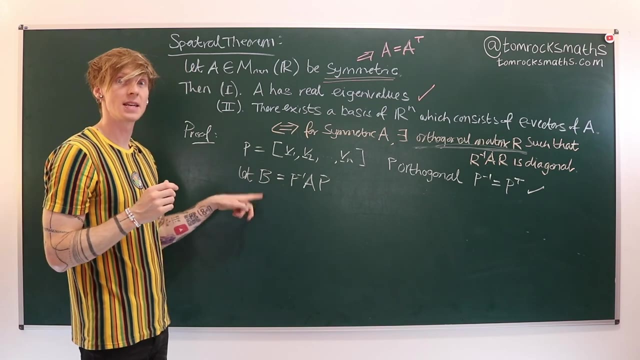 diagonal because p is definitely orthogonal. This is definitely true because these vectors, its columns, are orthonormal. It's an orthonormal basis that we constructed from Gram-Schmidt. So we know this is true, but we need to check that this is diagonal. So we want this. 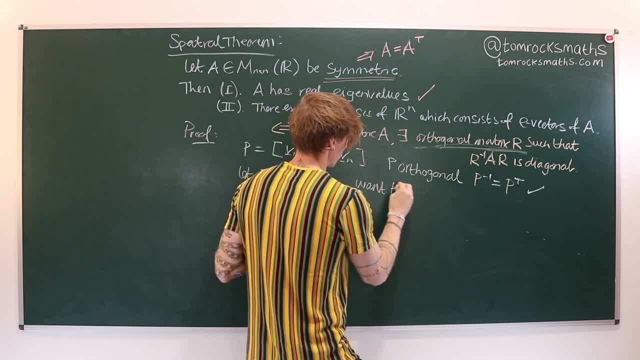 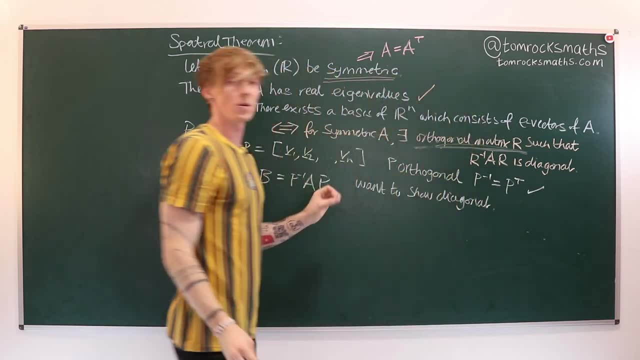 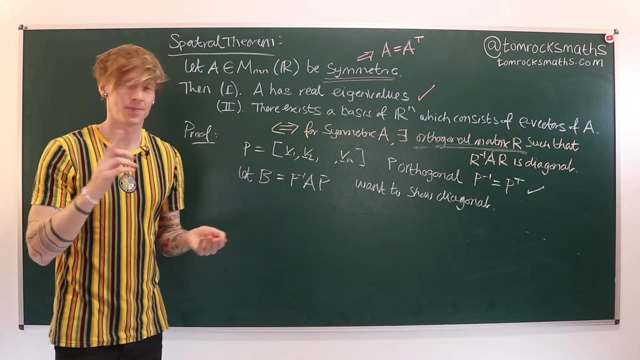 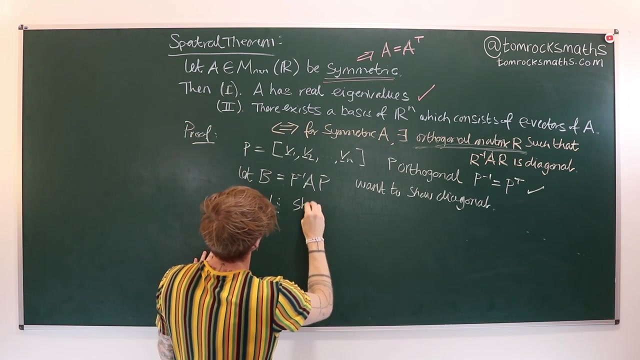 we want to show, want to show that this is diagonal. So, in order to do that, in fact, our first step is going to be to argue that b is in fact symmetric. So step one is going to be: show b is symmetric. Now, fortunately, we can just compute this: 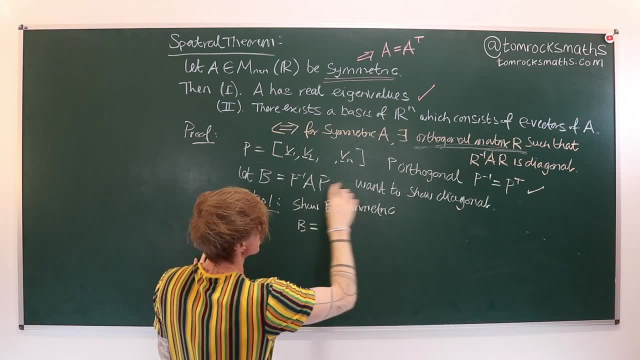 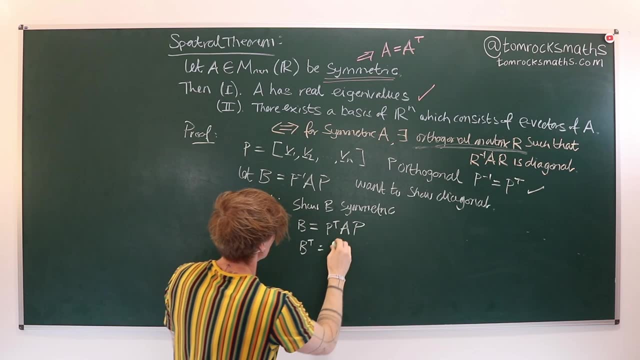 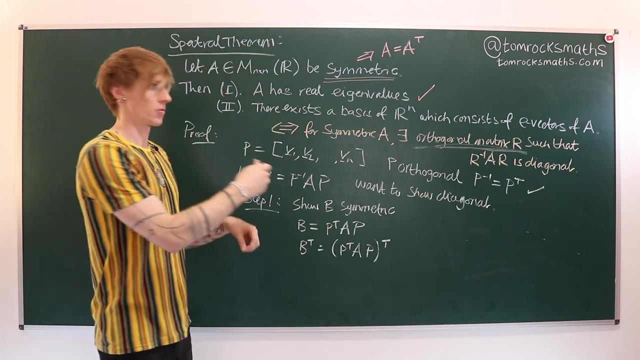 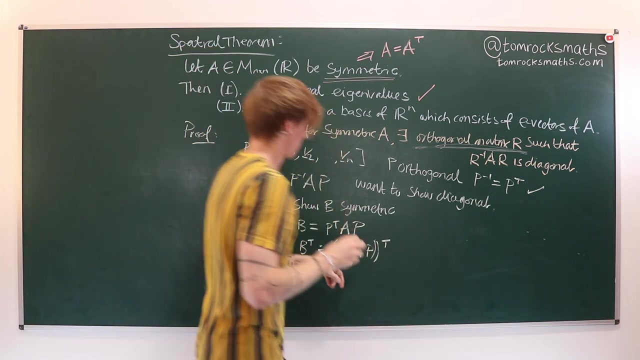 because we know that b is equal to p inverse, but p inverse is p transpose, so b is that? So if I calculate b transpose, then it's p transpose, A, p all transposed, and now sort of using the transpose expansion of a bracket if I write that as one factor. so if I call p transpose, 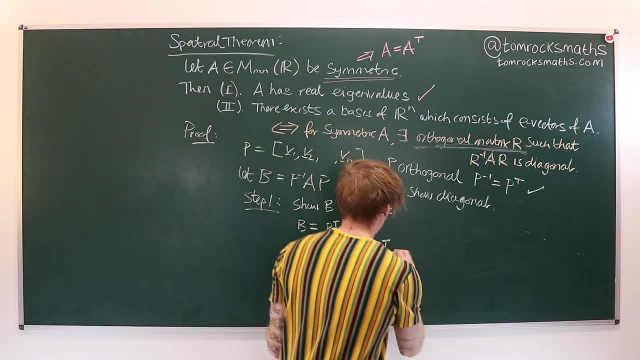 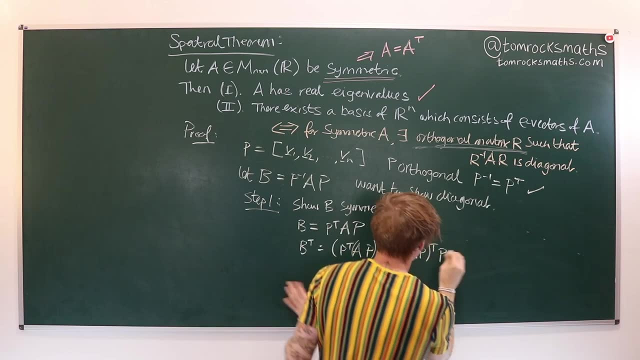 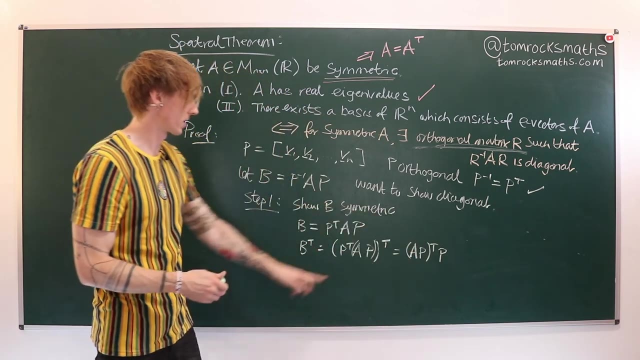 the first factor and A p the second factor. then transpose, law says that will be AP, all transposed times P, transpose, transpose. If you take the transpose of a transpose you get back P. So that's doing the first expansion of the three terms where I'm splitting them up like this. and now 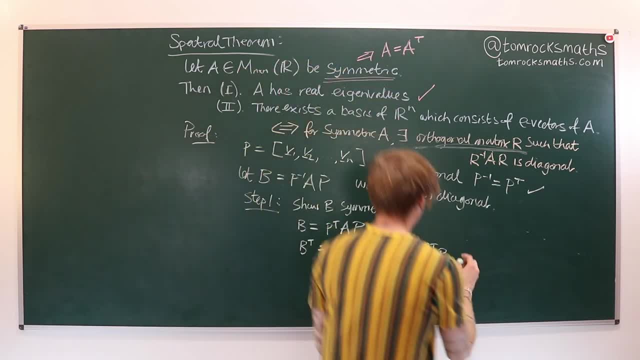 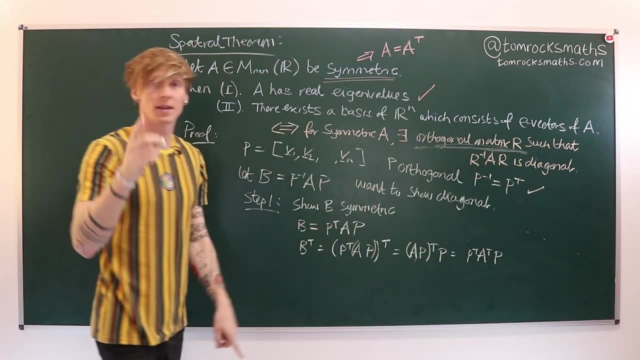 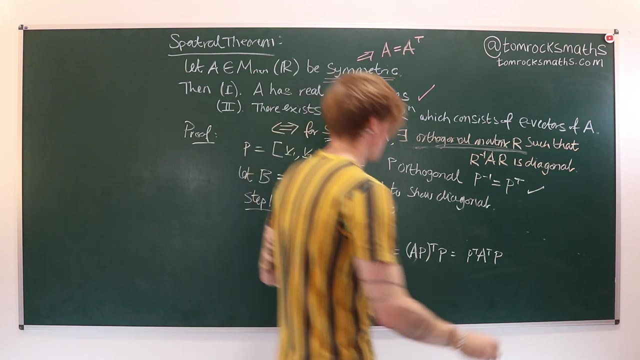 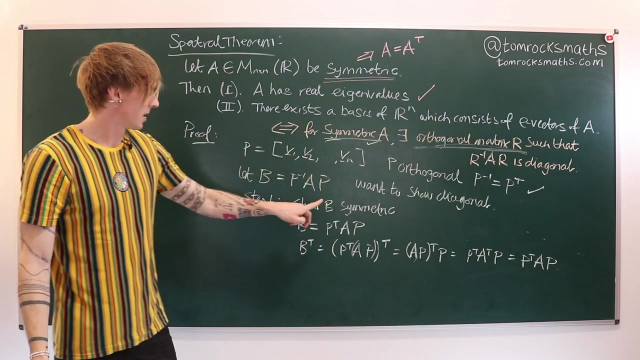 applying the transpose rule again to that bracket gives me P transpose A, transpose P. but A is symmetric- that thing that we always come back to symmetric A up here. I'm going to use that result now. A is symmetric, so that's actually P transpose AP. Okay, so we've shown that B is P, transpose AP B. 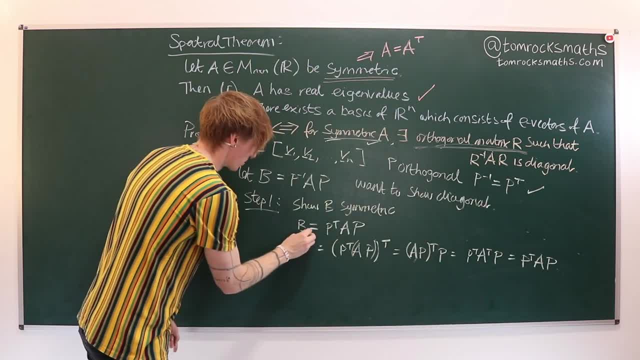 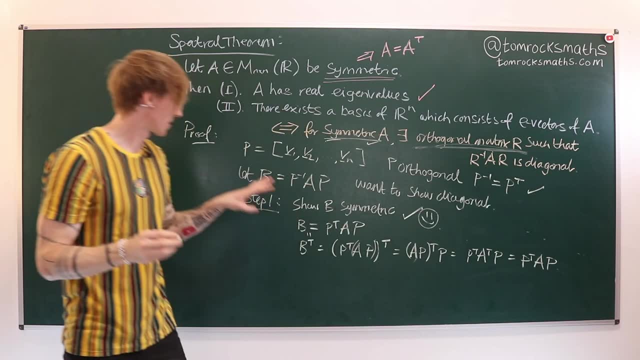 transpose is the same thing, so they're equal. therefore, B is symmetric. I'm going to put a tick and a smiley face- Subtitles by the Amaraorg community- because we've shown step 1 in terms of trying to show that B is diagonal For 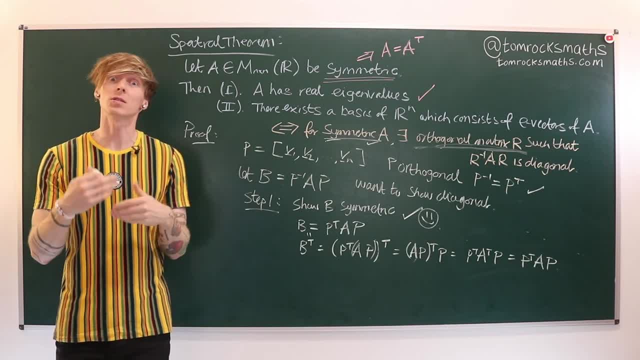 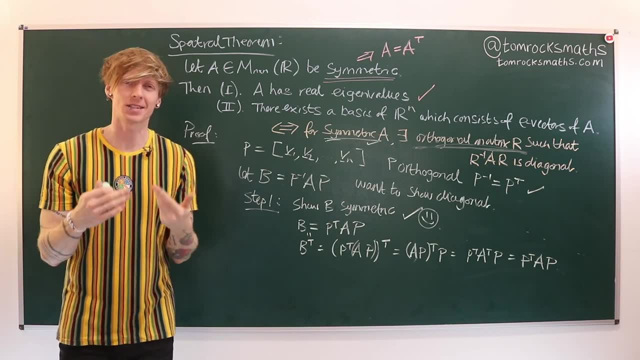 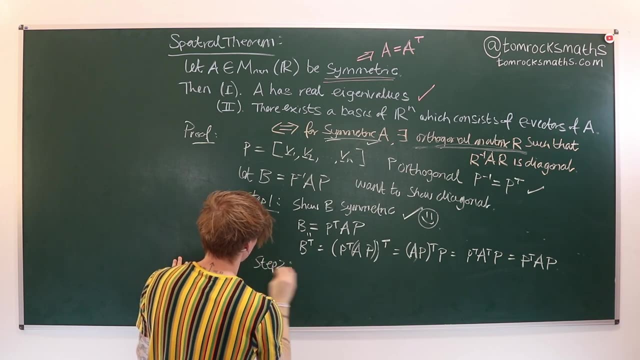 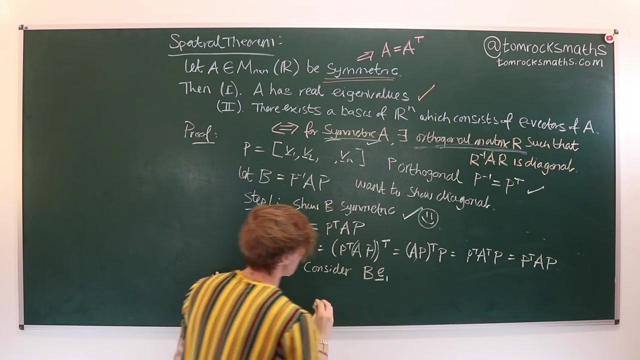 step 2, we are going to rewrite B in what is called block form to try to see the structure that this matrix must have and hope that it looks like it's going to be diagonal. So the way we do this is to consider the matrix B post multiplied by. 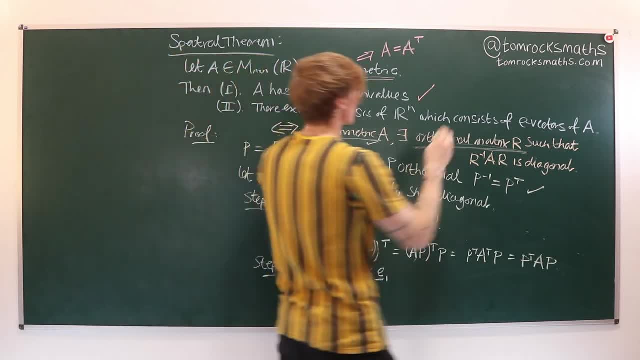 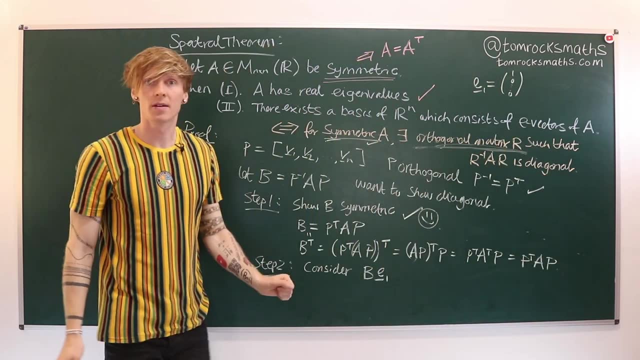 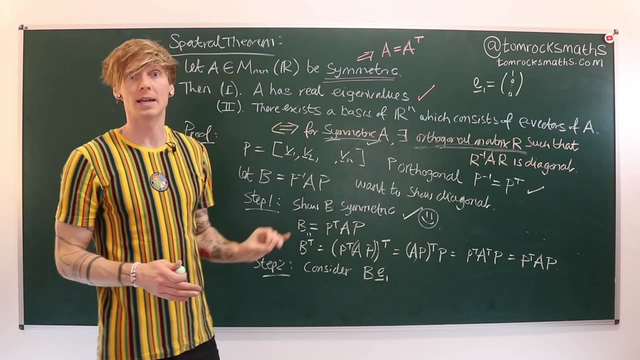 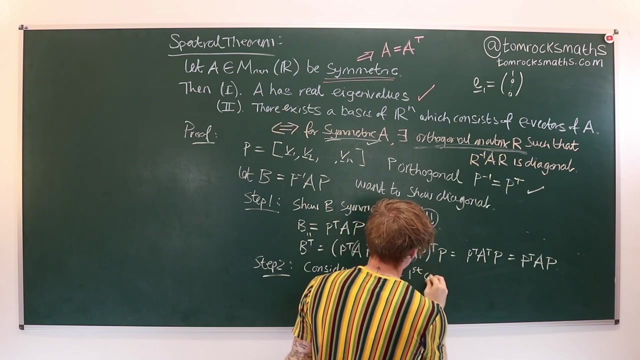 E1. Where E1 is the standard basis vector. so E1 would be one with zeros as a column vector. So if we take any matrix B and then we post, multiply by E1, this will actually give you the first column of your matrix B. and if you can't see this, 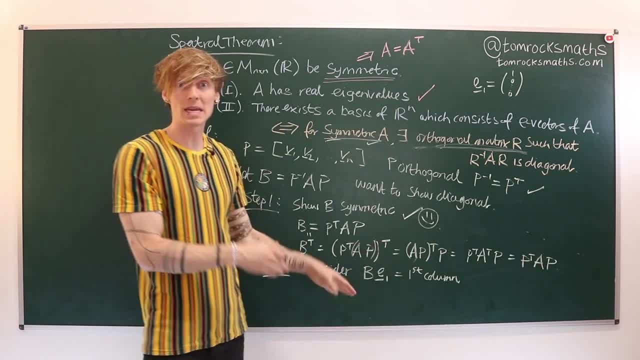 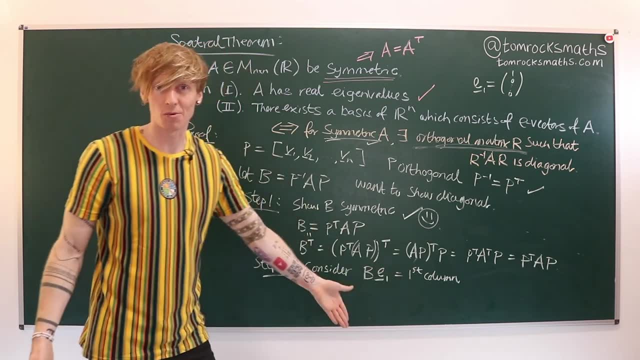 immediately. I do recommend: take a matrix B and multiply it by E1.. Take a matrix B, a square matrix, multiplied by your appropriately sized basis vector, standard basis vector E1, and you'll see, you do indeed get the first column of your matrix. 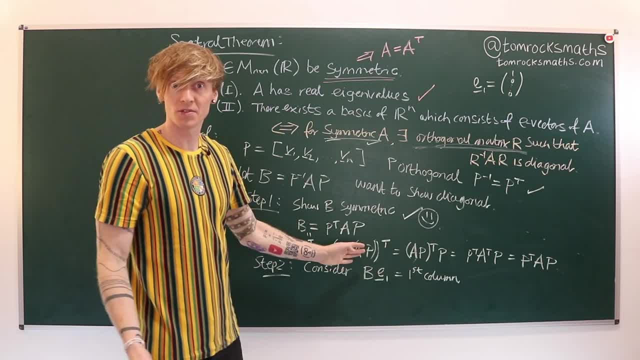 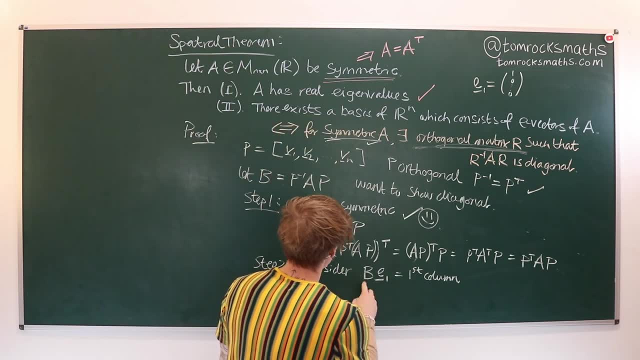 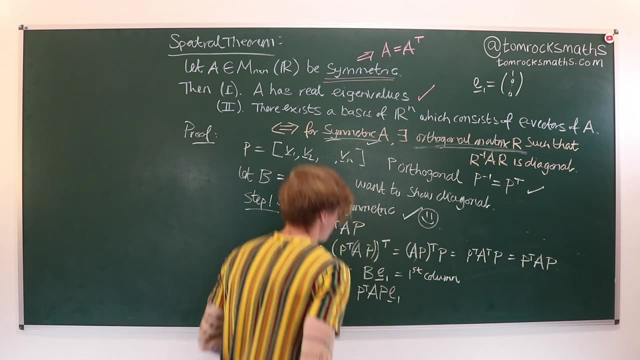 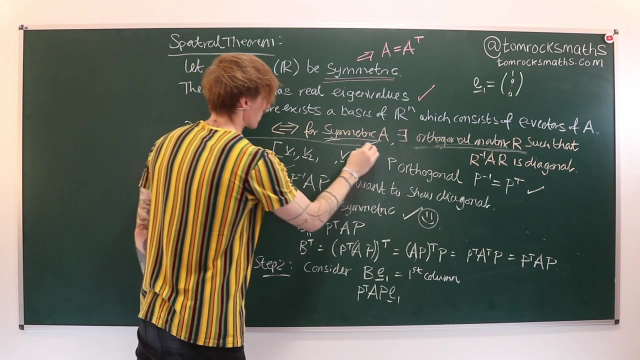 So the first column comes from this expression. Now we also know that B is equal to this. So we can actually say, well, B is P transpose AP. So this is P transpose AP times E1.. So we can actually say, well, B is P transpose AP times E1. But how did we define P? Well, P up here was given as a matrix where the columns are exactly the eigenvectors, the. 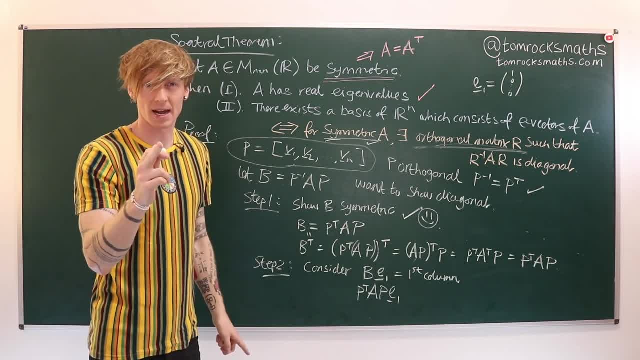 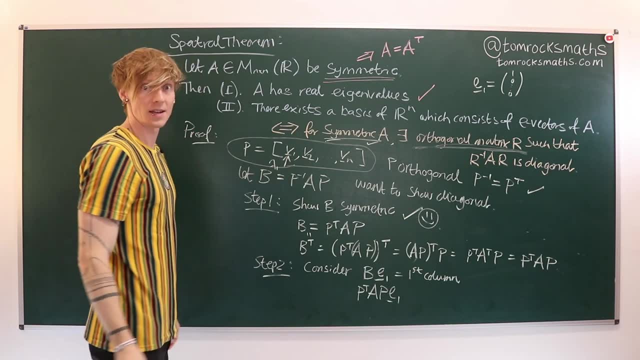 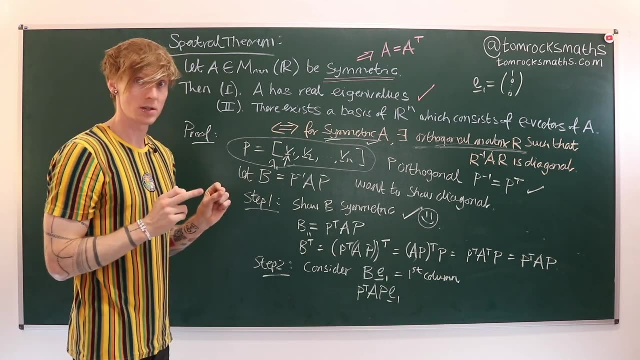 orthonormal basis. V1 is the eigenvector. That's the key thing. V1 here is exactly the lambda 1 eigenvector. That was how we started off this entire proof and this entire process. So what we can do is, first of all, P times E1 will actually give you V1.. 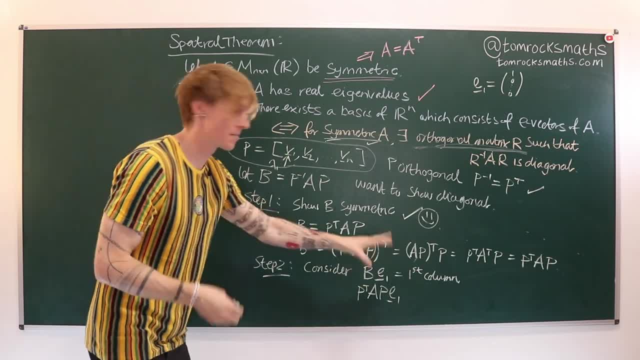 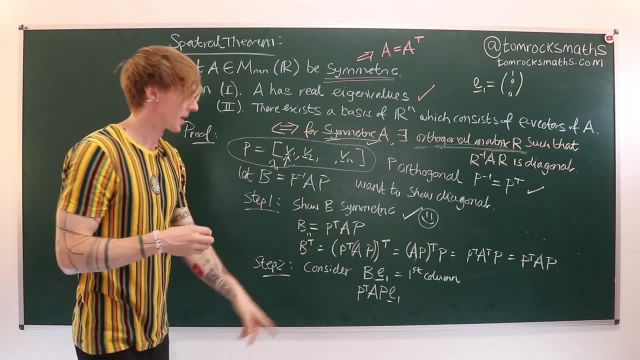 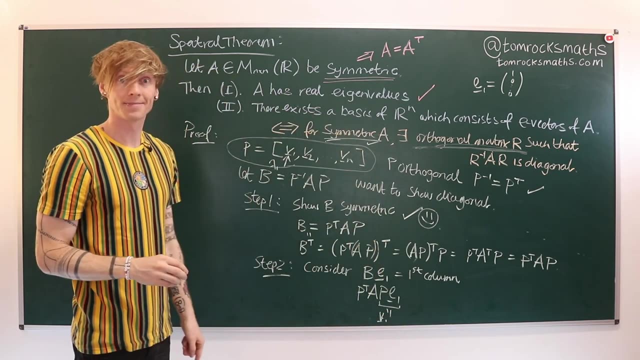 That's what's going to happen. Again, if you can't see that immediately, take your matrix P multiply by E1, you get the first column, just as we did for B. So the first column here that is V1, the first column of P. But that means this is equal. 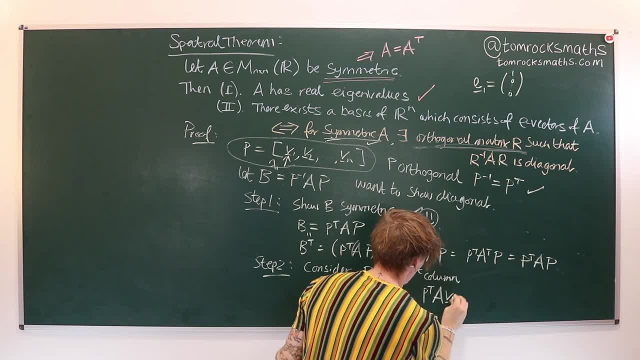 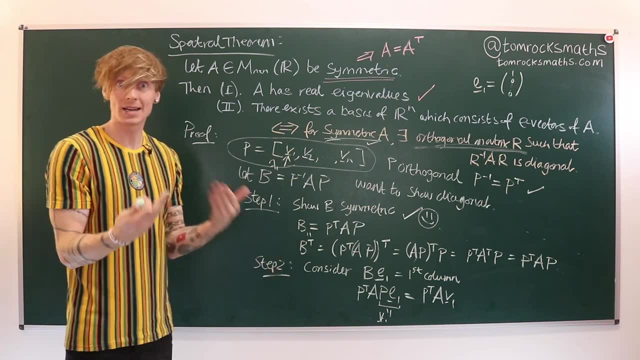 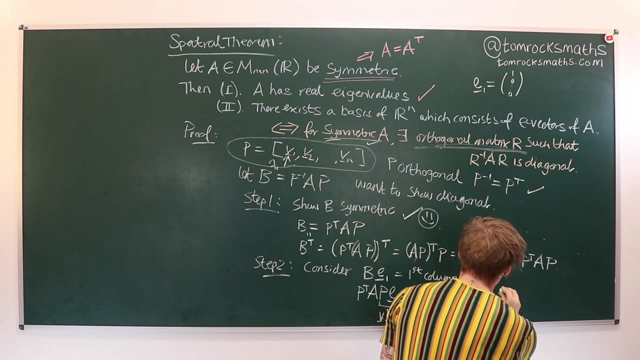 to P transpose AP. So I'm gonna say P transpose AP times V1. But then what is AP times V1?? V1 was actually the eigenvector for lambda 1.. So we can replace that by P transpose and then lambda 1 times. 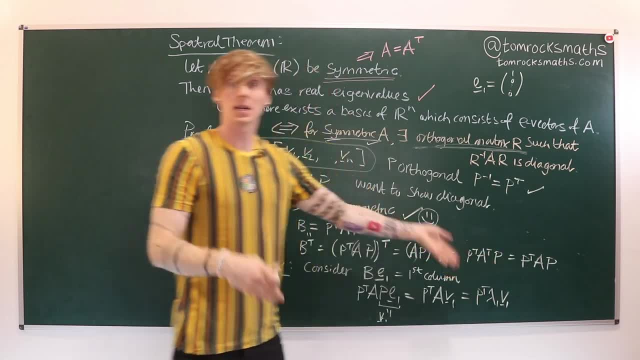 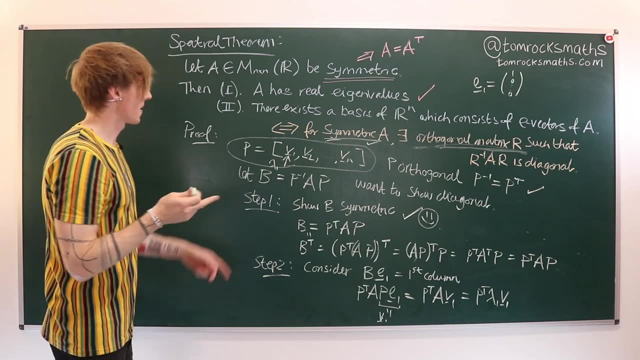 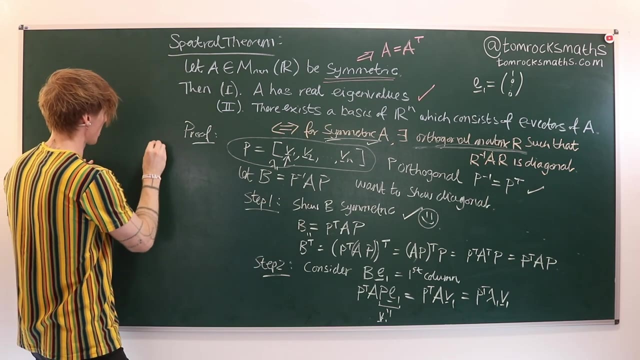 V1. Now lambda 1 again can come outside of that product because it's a matrix and a vector and a scalar. so we take lambda 1 outside And then if we have P transpose, multiplying v1. So p transpose, if I write it over here, is going to be it's going to have the first row. 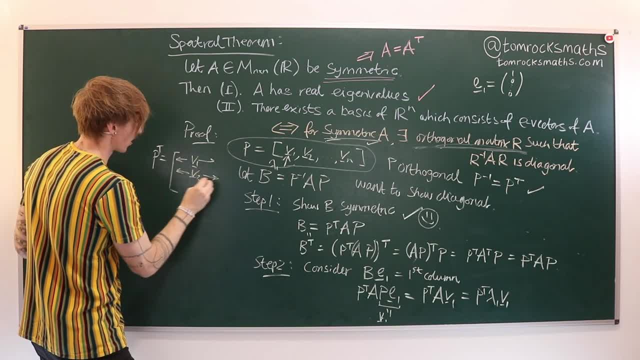 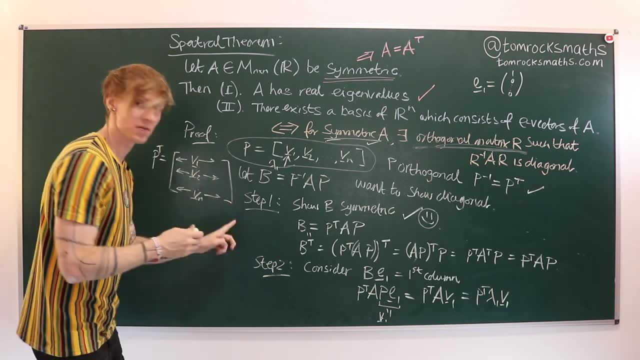 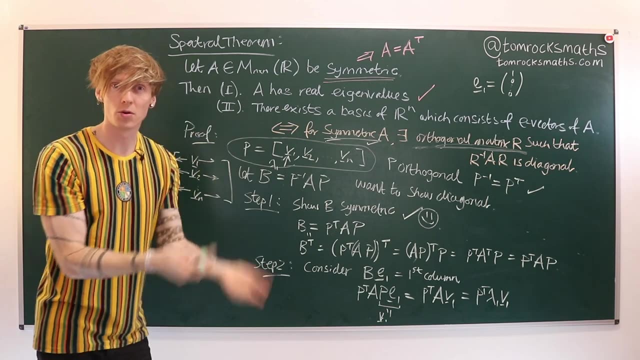 as v1, then v2, and the second row down to vn. So when we multiply this by v1,, you're going to get a v1 dotted with a v1,, which is 1, because it is orthonormal. All of these are orthonormal. 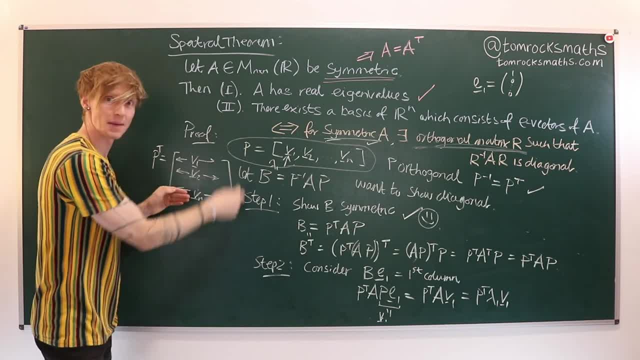 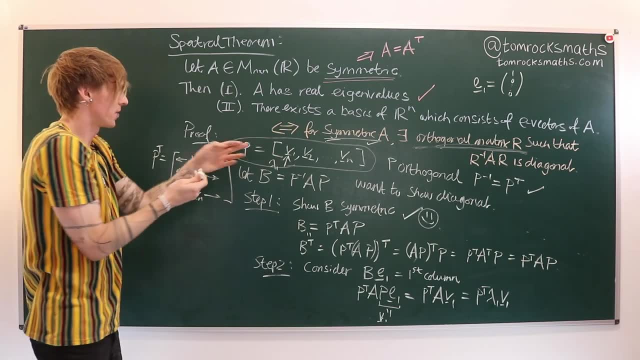 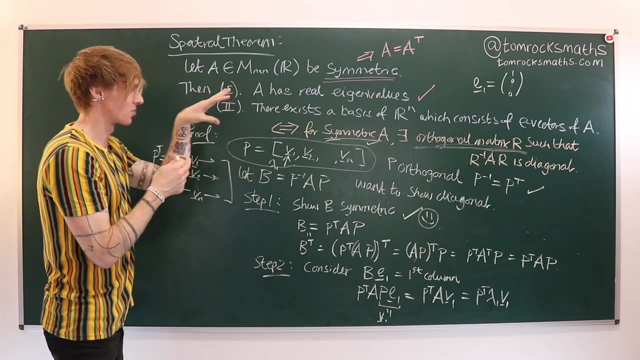 really important. And then when you do the second row times v1,, you've got v2 dotted with v1, but they're orthogonal. they're orthonormal. So if you dot any of these with any of the others, you get 0.. And this is where the orthonormality is really really important, because p transpose. 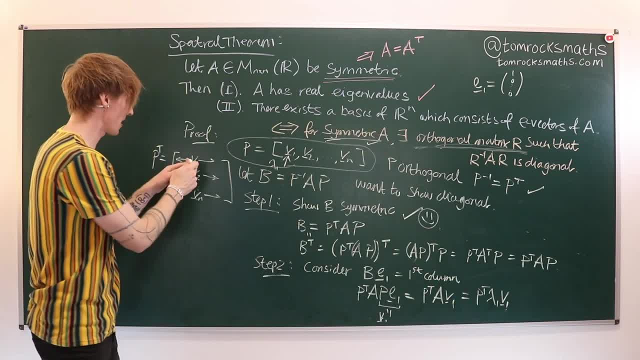 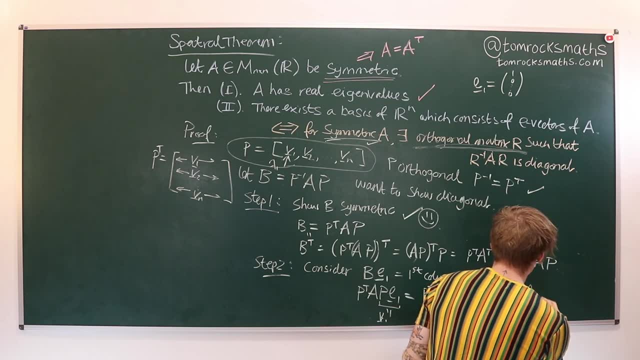 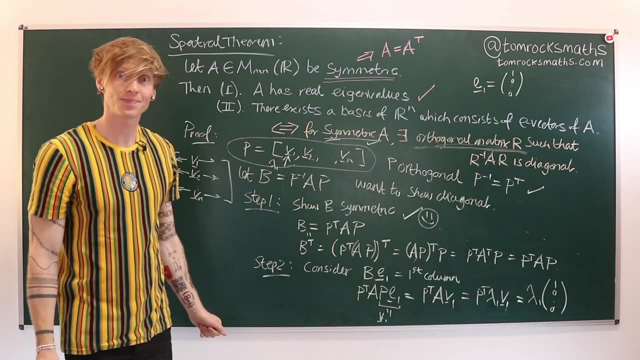 times, v1 is literally only going to pick out that first entry and is actually just going to give you the standard basis vector. So you have your lambda 1, and then you have back e1, or 1, with a load of zeros. So we can see, very importantly for our proof here- we can see: 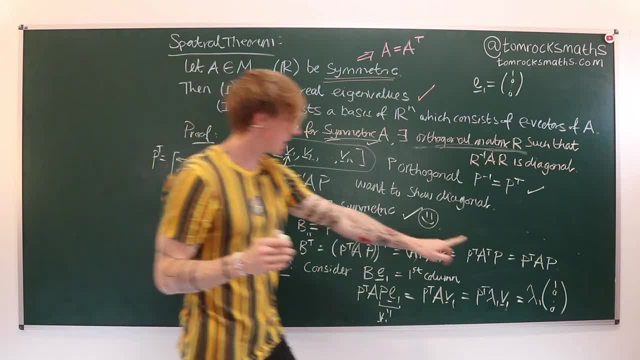 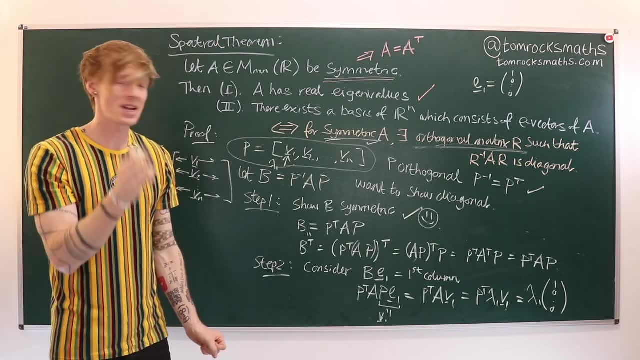 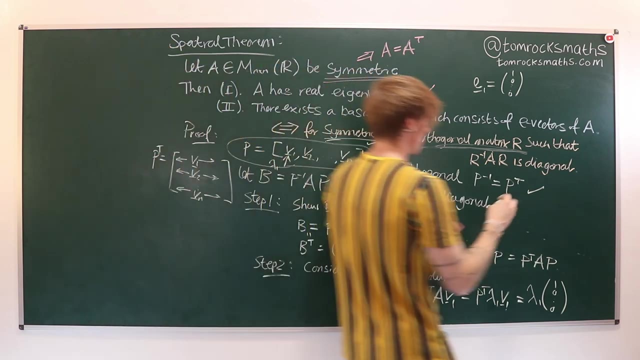 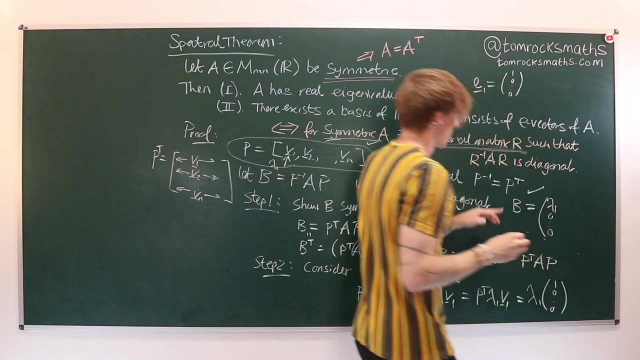 that the first column of B is going to be lambda 1 in the top entry and zeros all below that. Now, since the matrix is symmetric, we showed that B was symmetric in step one. we know the first column. the first column is lambda 1, 7the one人. 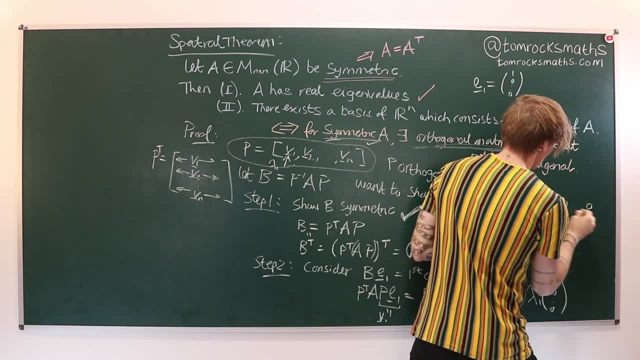 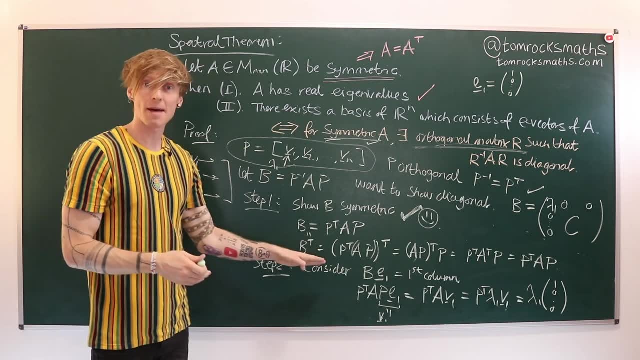 the first column is lambda one with zeros, But because it's symmetric when we take the transpose, we have to get b, That's the first row has to also contain those same zeros, and then i'm going to call this thing c. 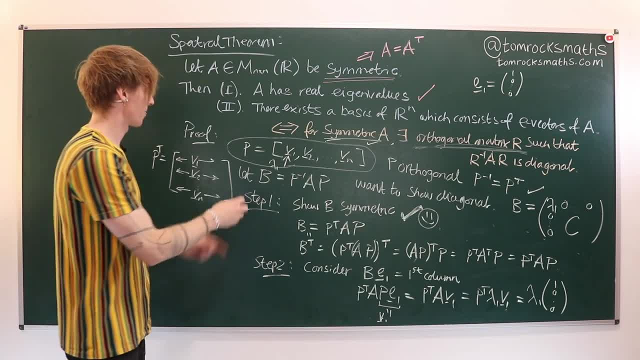 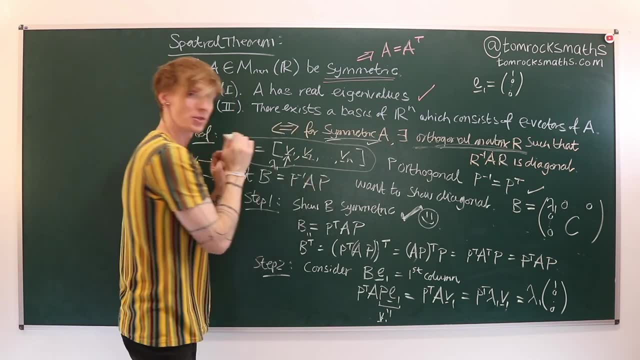 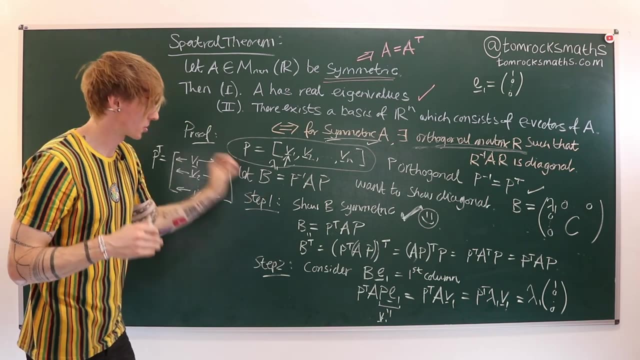 What we've been able to show is that, by defining this matrix B, taking our orthonormal basis, pre-multiplying by its transpose, post-multiplying A by that matrix, we've been able to get this new matrix B And we've been able to show that B has this form. 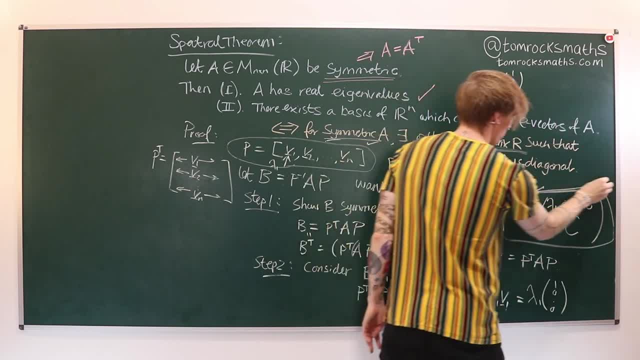 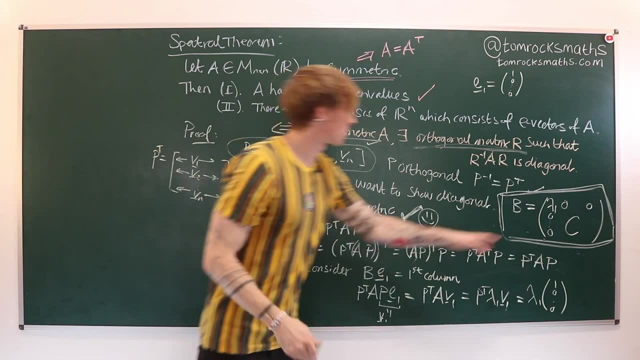 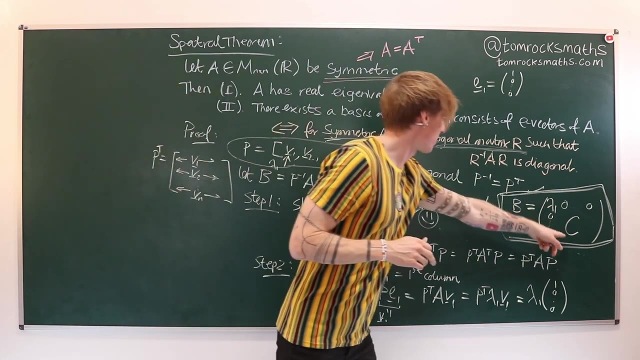 So the first row and the first column are satisfying the need to be diagonal. However, we don't at the moment know anything about C except its size. So the matrix C is M minus one, by M minus one, It's dimension one smaller. 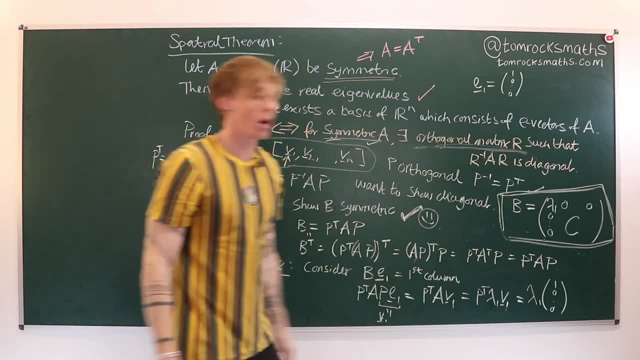 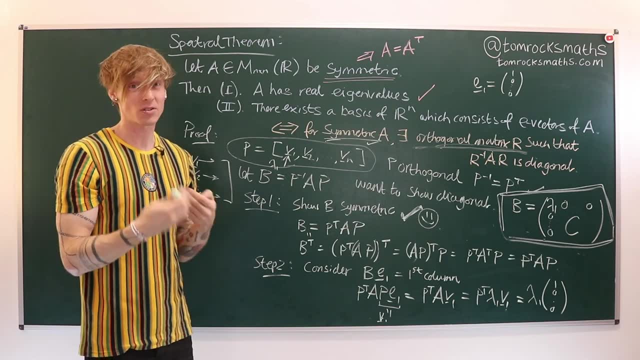 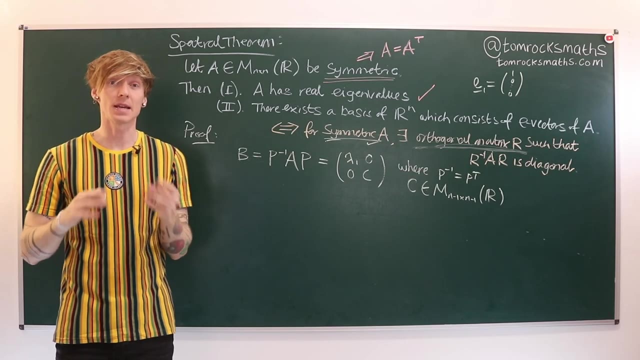 And our next trick is going to be: can we show that C is also diagonal, or can we remove one from its dimension? And that, to me, is crying out for a proof by induction. The final step of our proof by induction Of the spectral theorem is to use induction on the dimension n. 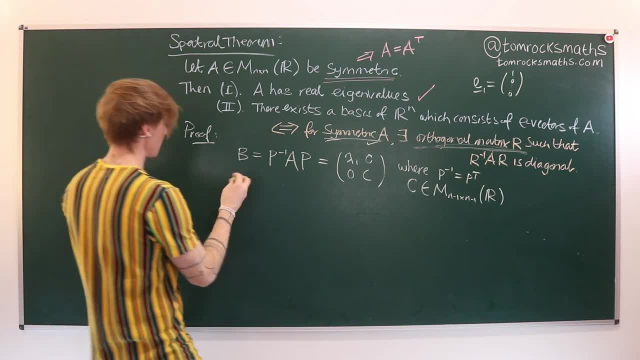 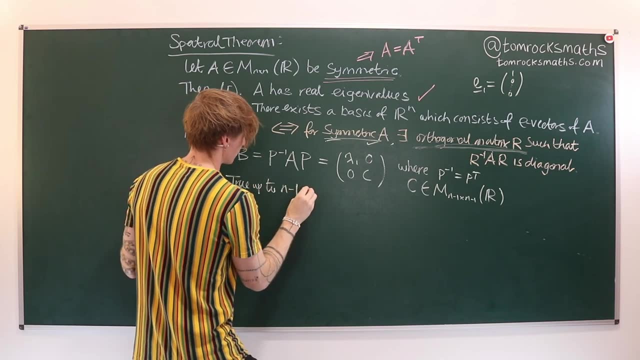 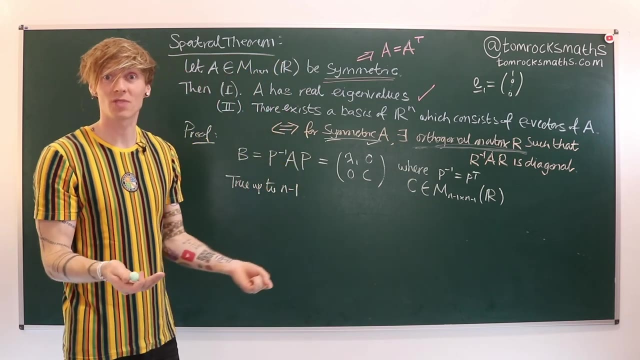 So if by our inductive hypothesis we assume that it's true up to n minus one dimension, then we have a matrix C which is M minus one, by M minus one, And it's real and it's symmetric. So by the spectral theorem that means: 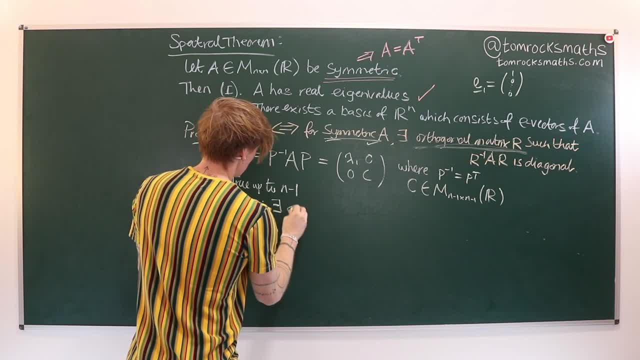 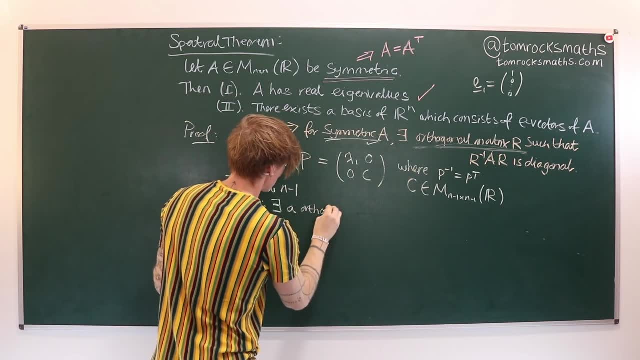 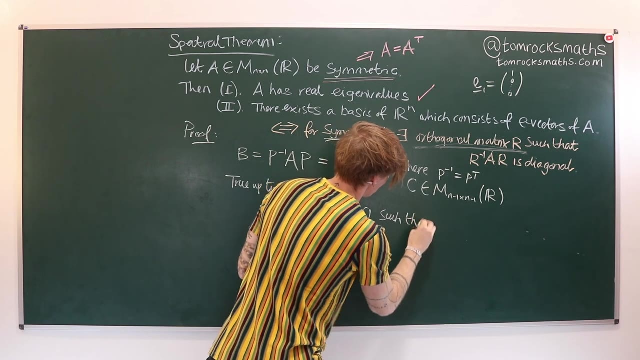 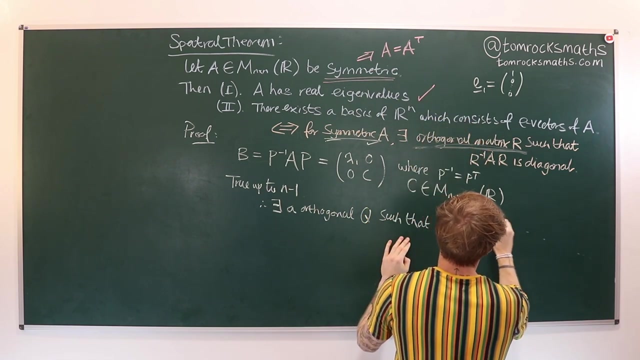 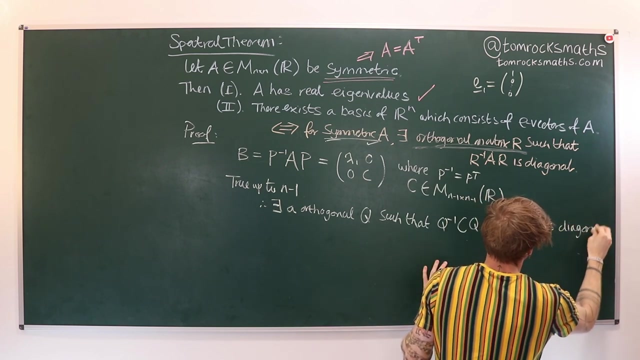 That there exists A basis. so therefore there's just an orthogonal matrix. There's this orthogonal Q, such that Q minus one Times C times Q equals D, which is diagonal. So D is being used here to emphasize the matrix is indeed diagonal, zeros everywhere. 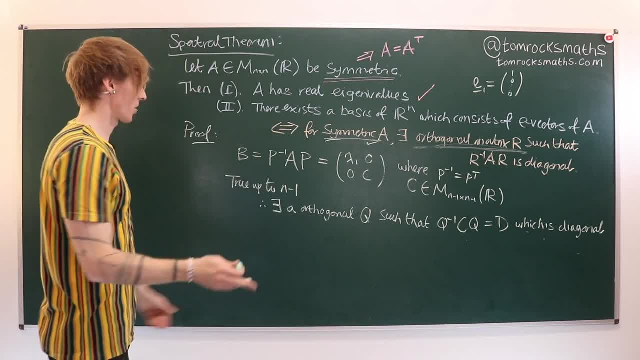 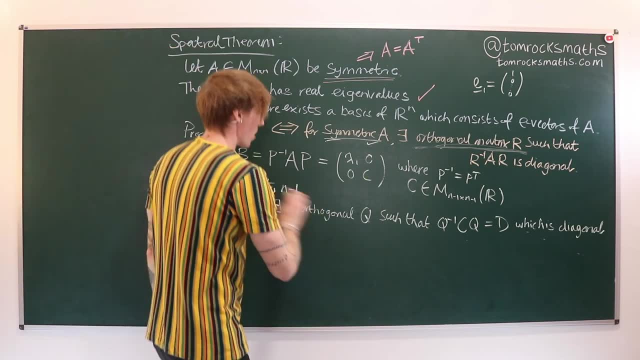 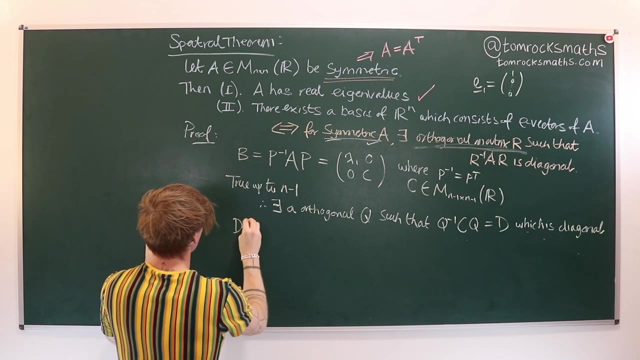 Just that main diagonal that has entries. So this is our inductive hypothesis. Now, with this assumption, we want to show that this is true for our end by end matrix that we have up here, And the way we do this is we define: 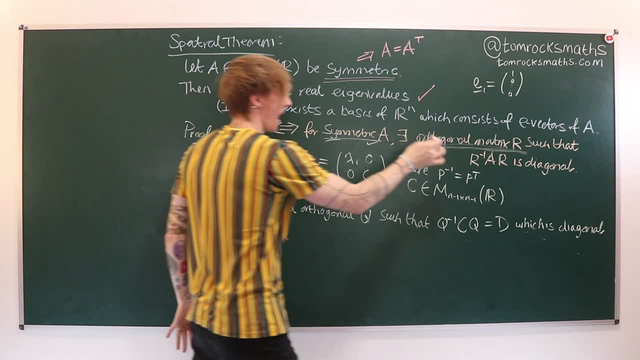 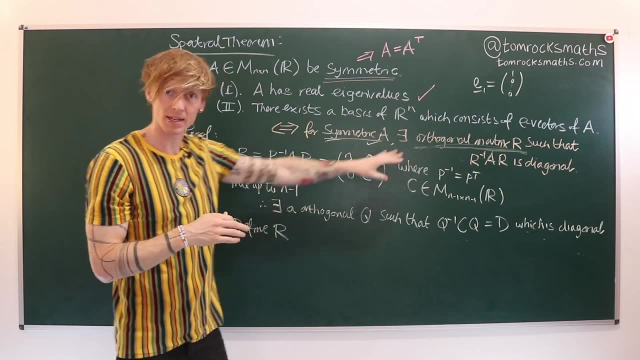 Are The matrix now the actual one that we're trying to get, So, as I mentioned earlier, very similar to P, And that's why we were calculating the same kind of things. But now we have our actual matrix, R, So we define this to be: 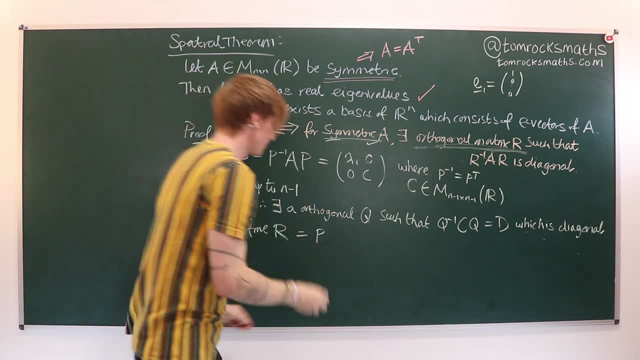 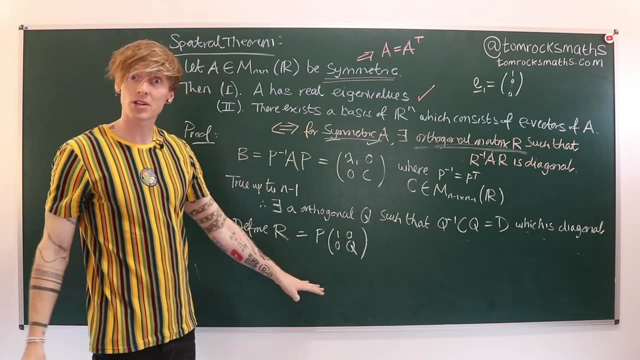 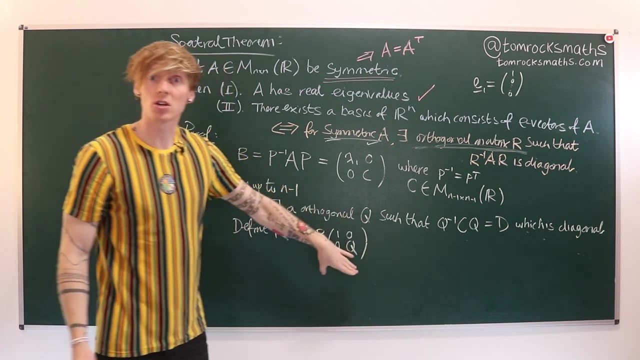 Our matrix P that we found earlier, Multiplied by one zero zero, and in our matrix Q, So I'm using block notation again. This is a row of zeros and a column of zeros, Apart from the leading entry one, And then we have a matrix Q in this matrix. 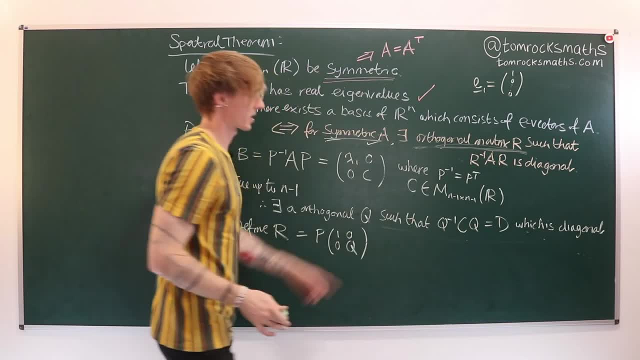 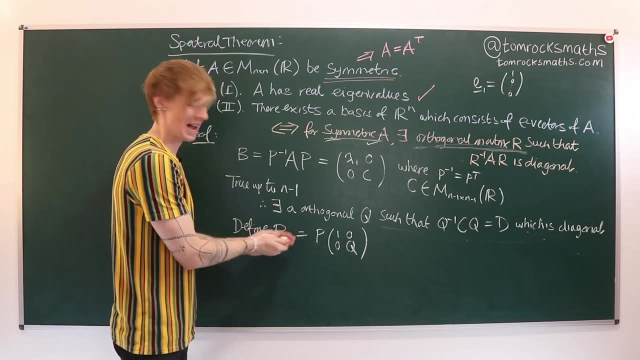 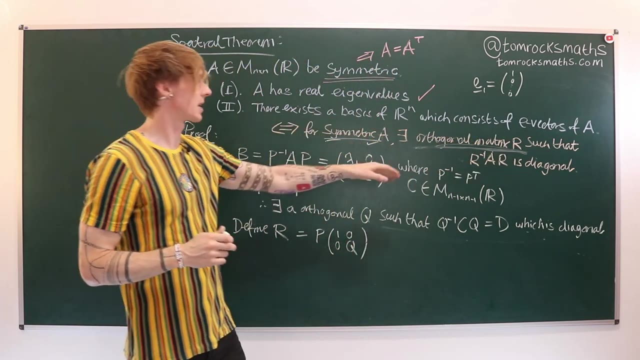 Bottom corner, where Q is exactly This matrix up here. Now there are two final things that we have to show are true for our matrix R, as defined here. The first thing is that R is orthogonal And the second thing is that R minus one AR is diagonal. 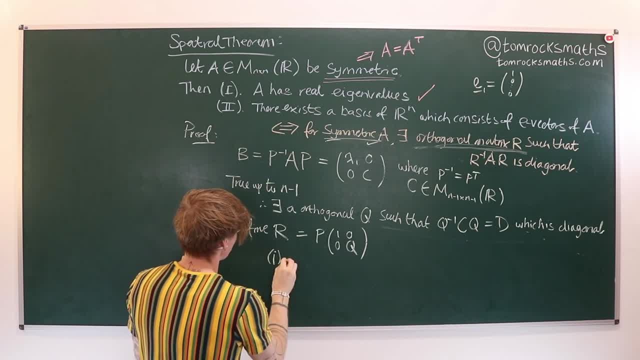 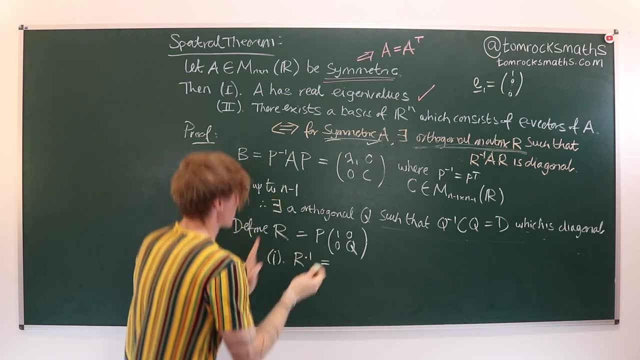 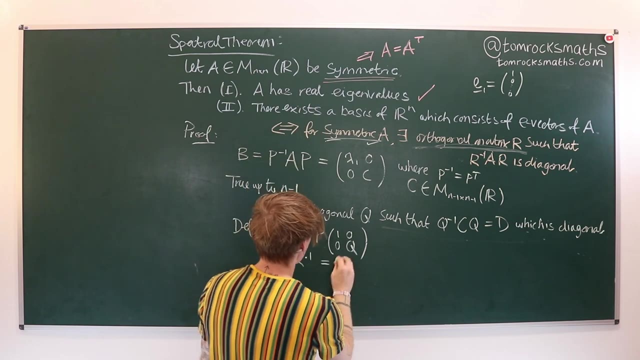 So first thing, Part one, We want to show that R is orthogonal. So let's compute R inverse, So it's a product. So if you take the inverse of a product, Swap the orders And take those inverses, So it's going to be. 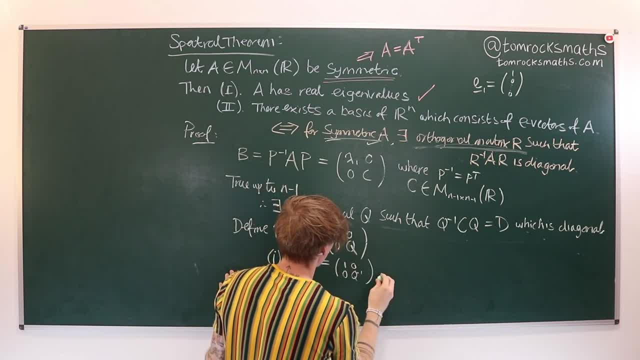 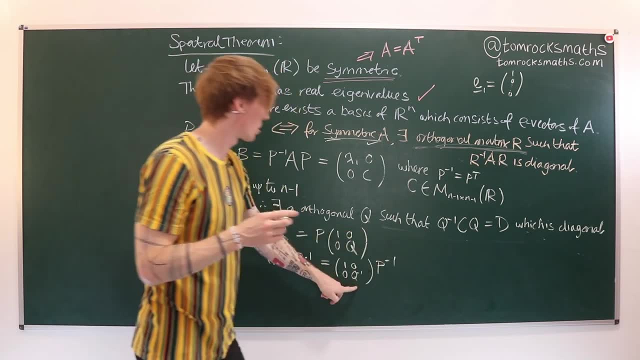 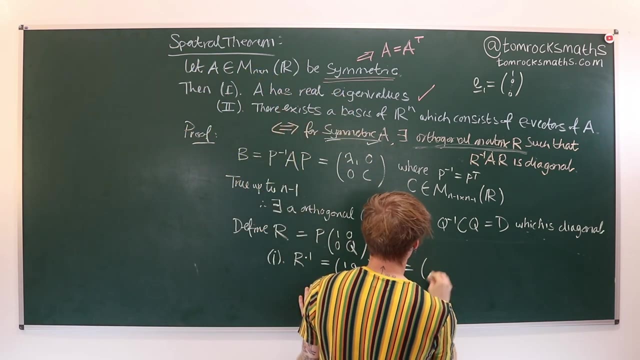 One zero zero Q inverse Multiplied by P Inverse. Now We know that both P and Q are orthogonal, So their inverses are their transpose. So this is in fact Equal to One zero zero Q transpose. 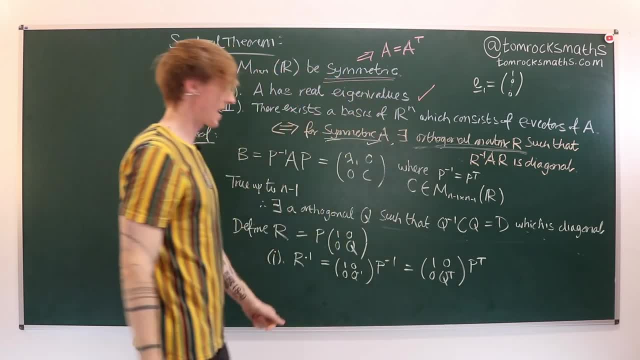 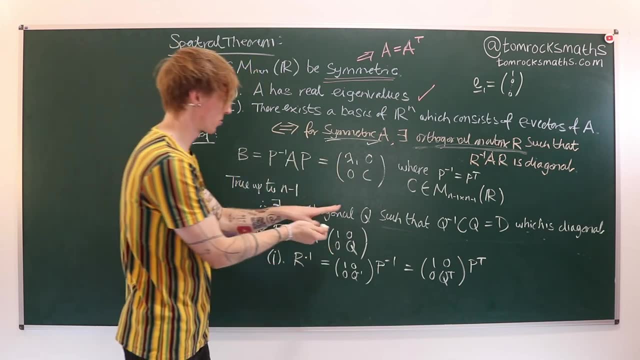 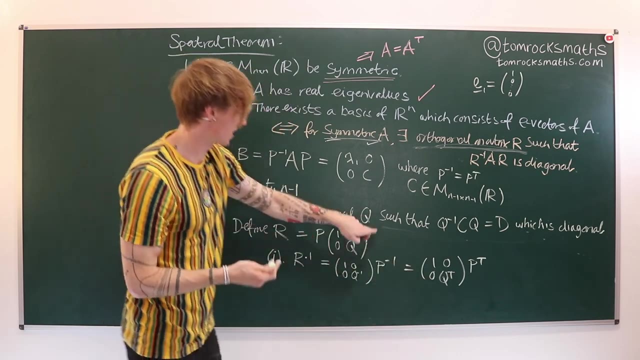 Or multiplied by P, transpose. And if I now compute, R transpose, So this is R, It's a transpose of a product, So you transpose. The second one goes at the beginning With a transpose- Exactly that, And then the first one goes to the end. 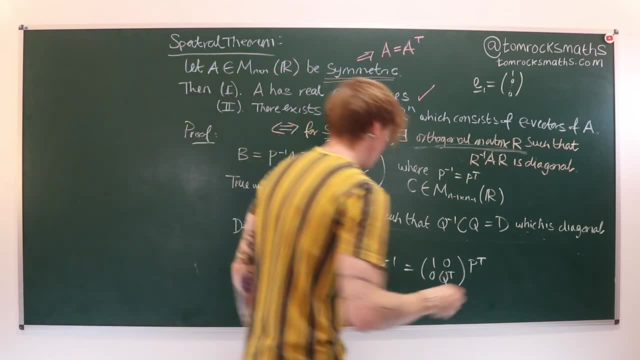 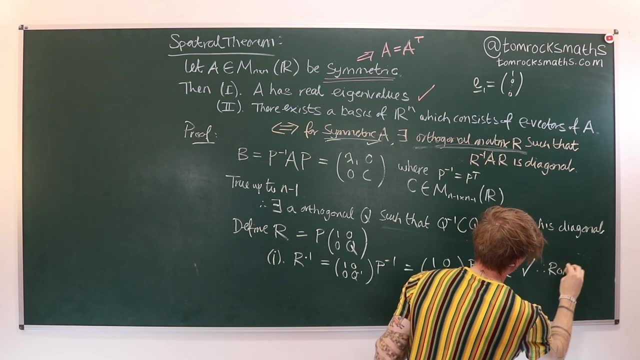 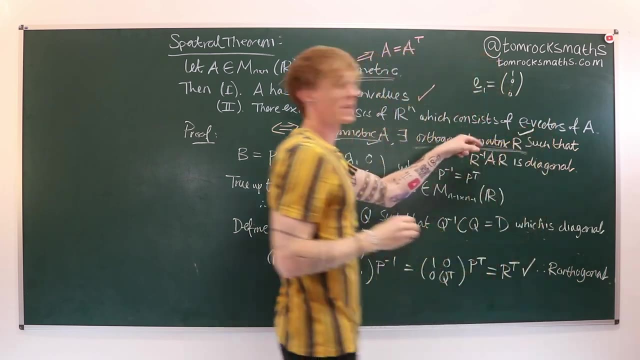 With a transpose Exactly as we've got. So this is R transpose. Okay, So that works. So therefore, R is orthogonal. So that's the first thing Shown to be true up here, That R is an orthogonal matrix. 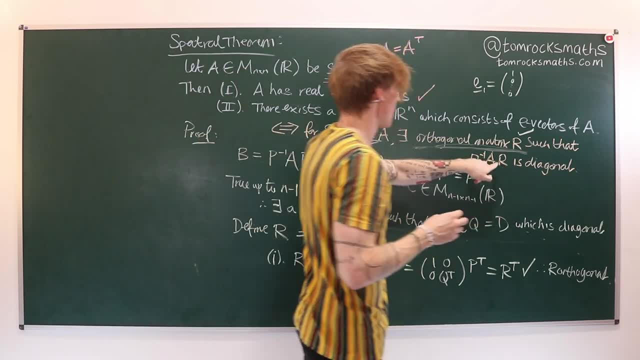 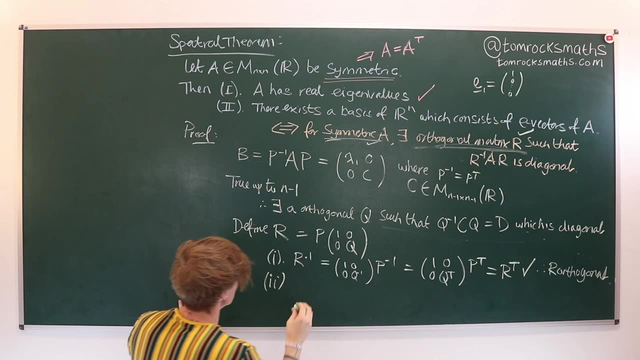 And now we need to compute R minus one A R To show that It's diagonal. So that's going to be part two down here Is to say: Okay, well, let's compute R minus one A R. Now we've already shown that R inverse. 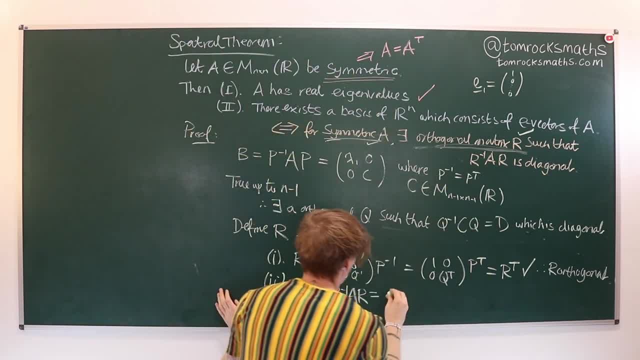 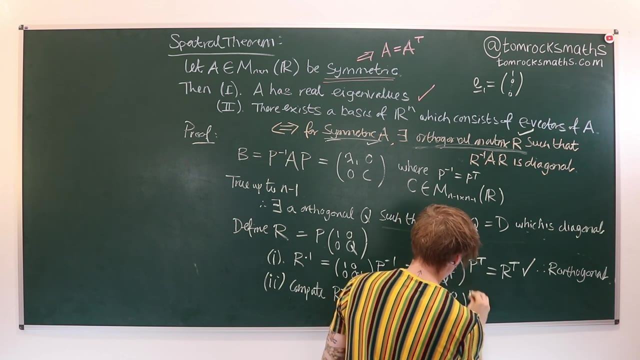 R minus one Is the transpose, So that's R transpose A R. But what is R transpose? We calculated it here, So that's One zero, zero Q. transpose Times P. transpose Times A Multiplied by R. 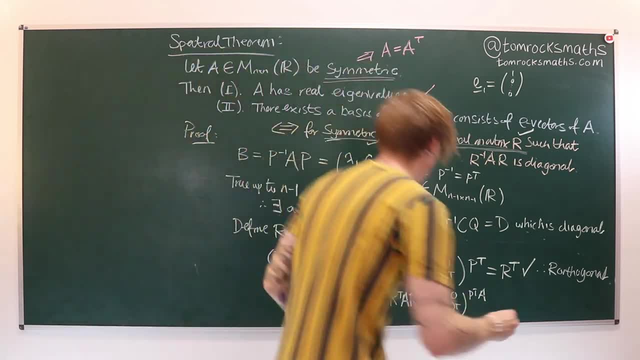 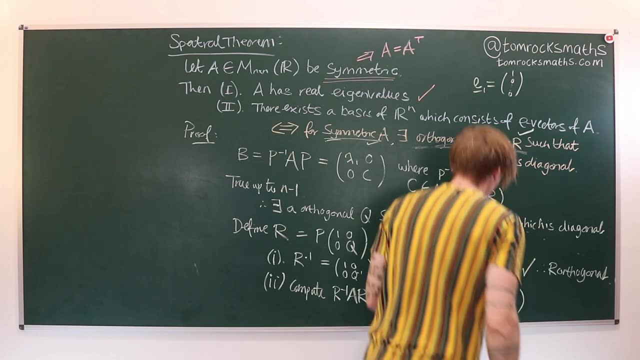 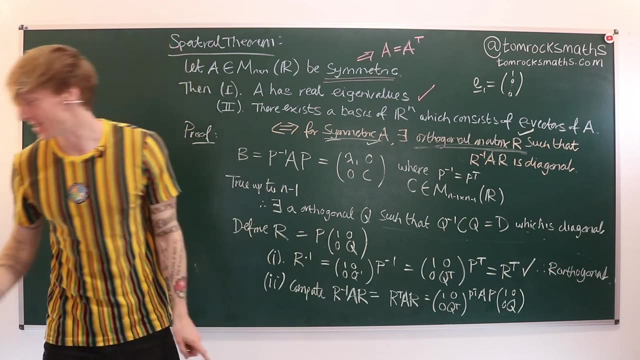 But R is P Times this block matrix. So we got a P Times One Zero zero Q, Zero zero Q. And now For the clever part. So this looks a little bit of a mess. However, We're going to get a different. 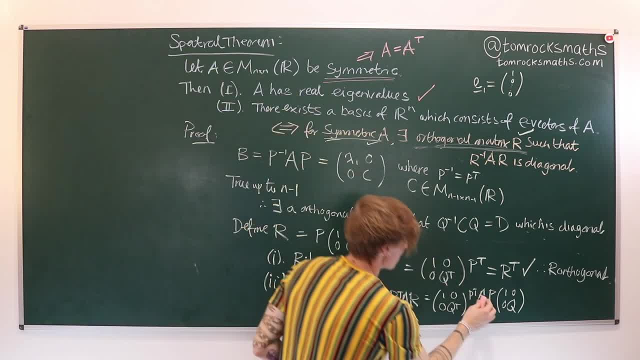 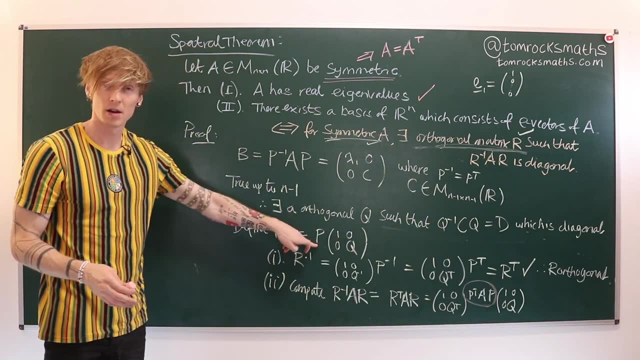 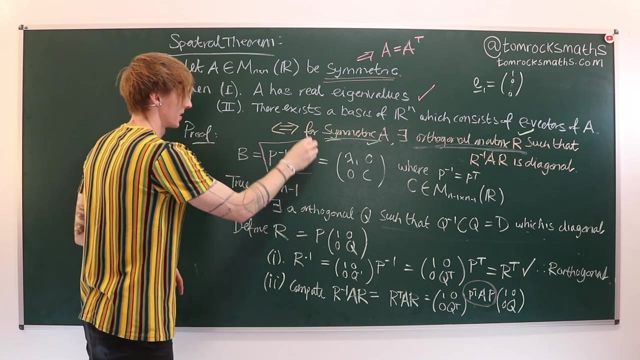 Color of chalk to emphasize this. What we've got in the middle Is P transpose A P, And this comes from how we defined R With the matrix P at the beginning, Because P transpose A P Is exactly This. 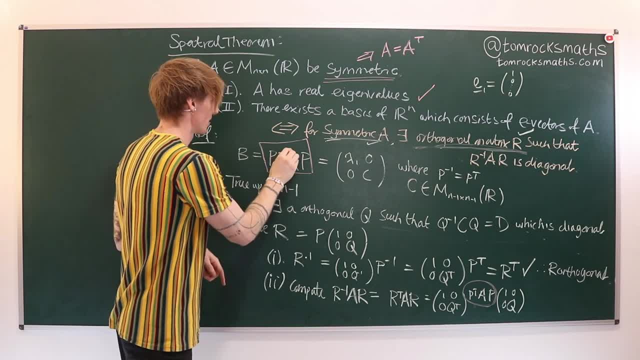 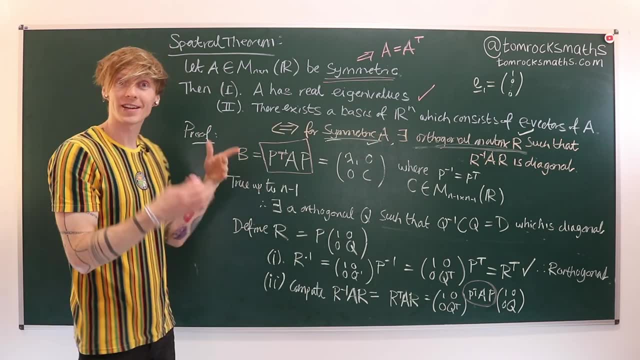 It's equal To B Because P inverse. up here, Remember, is P transpose. So This Is our matrix B. What is our matrix B? Our matrix B Is this thing Under one zero, Zero C. 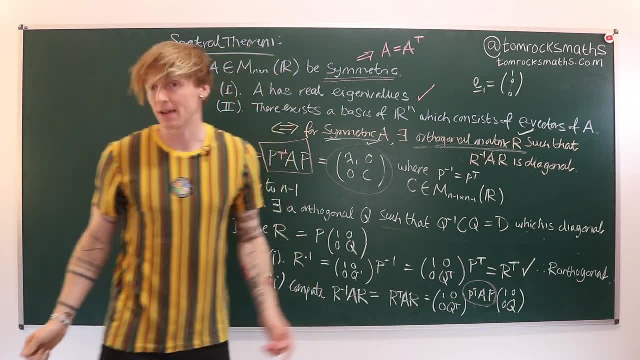 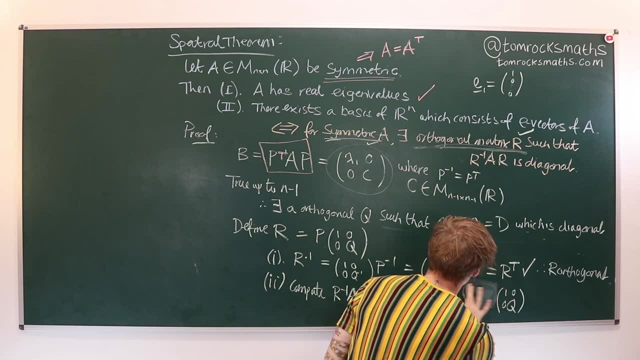 So We substitute that in. I'm probably going to have to rub this off, Substitute it in. here We're going to have a product Of three matrices Where This one goes in. So Lander one, Zero, Zero. 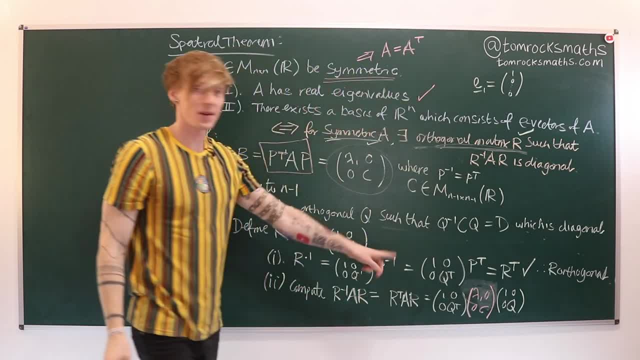 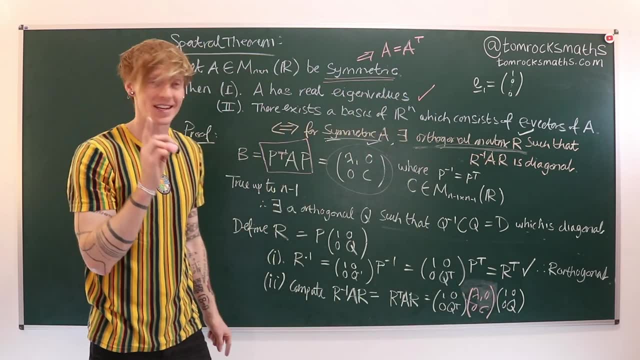 And C. Now If you expand out These matrices Because Of the simplified First columns In all of them With all of the zeros, This is just going to give you Lander one, That first column, Zero. 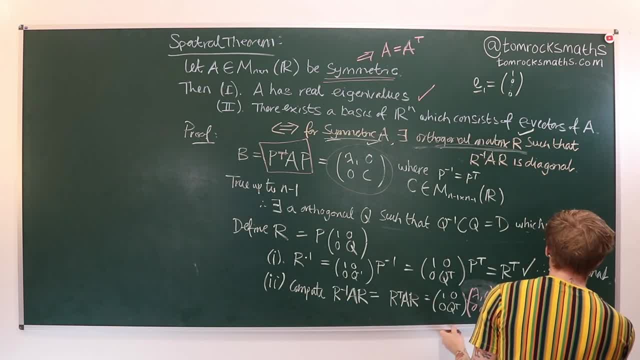 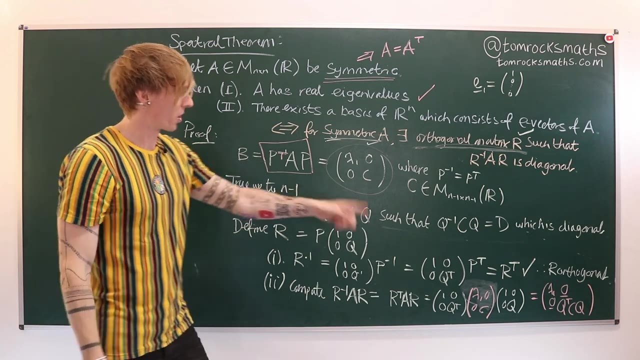 Everywhere else, Zero, Everywhere else. And then you've got Q Transpose C, Q Transpose C, Q. Now, What did we say? Q Transpose, Which, remember, is Q Inverse. 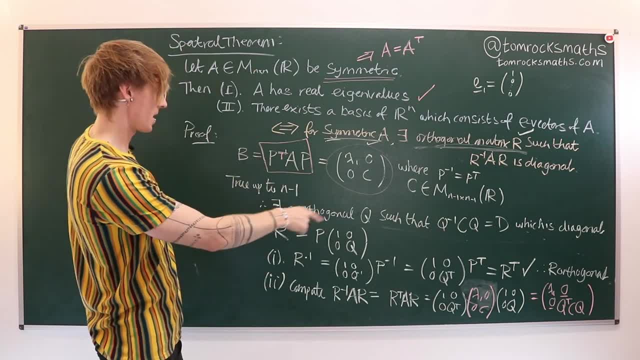 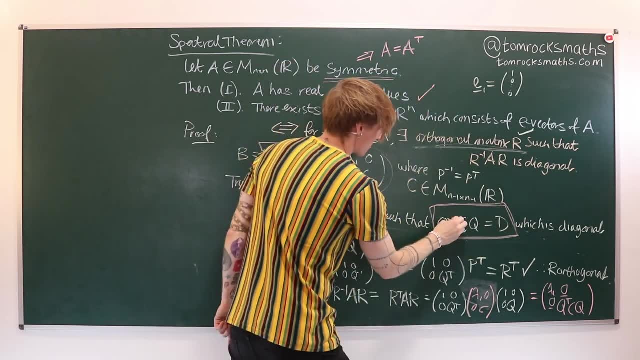 What is Q Transpose, C, Q Equal to Up here We said it was given By our diagonal matrix D. So This, Remember, Inverse is Transpose. This Is our diagonal matrix. 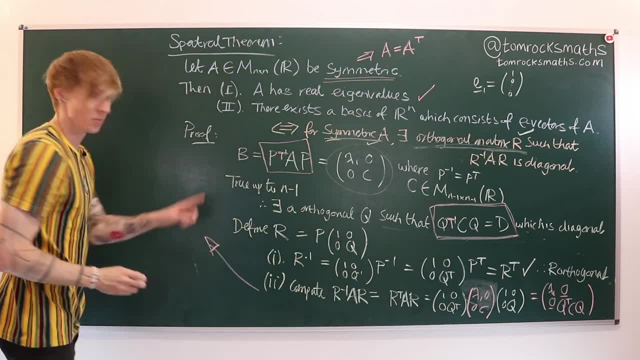 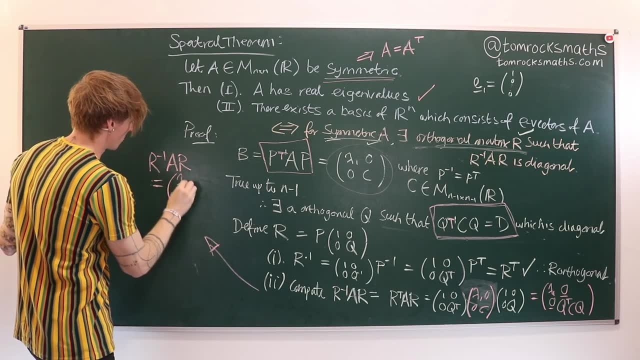 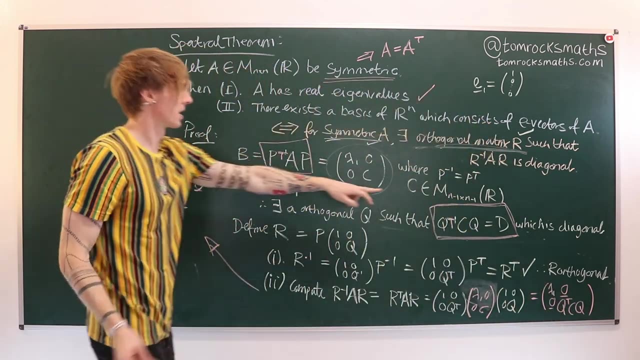 D. So D Goes down there And we have shown R Minus One A. R Is equal to Lander. one Zeroes Zeroes. And then Q Transpose C Q. 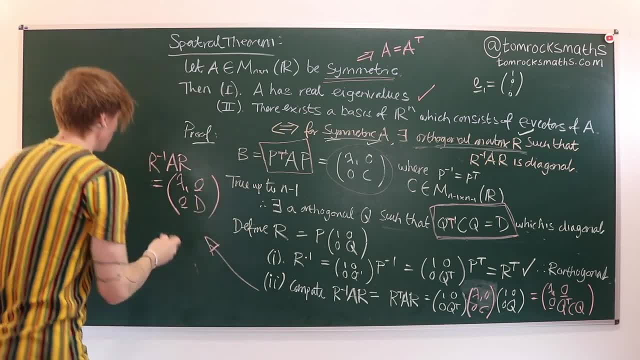 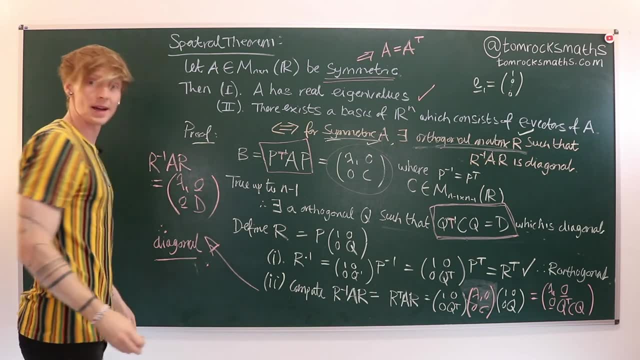 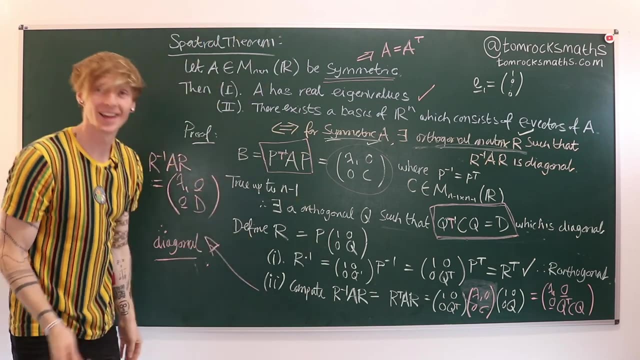 Is the same as Q, Inverse C. Q Is diagonal, matrix D. So We've shown Therefore Diagonal, And We've completed True, By induction. We've completed So The Whole. 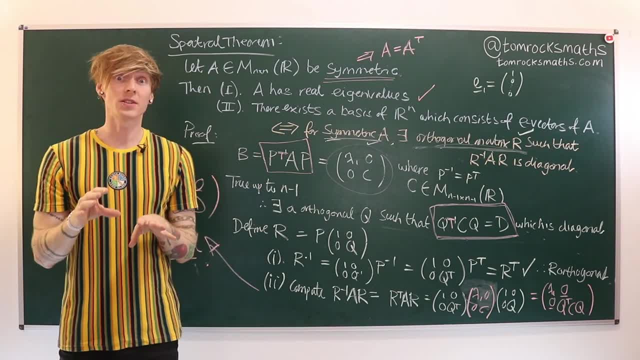 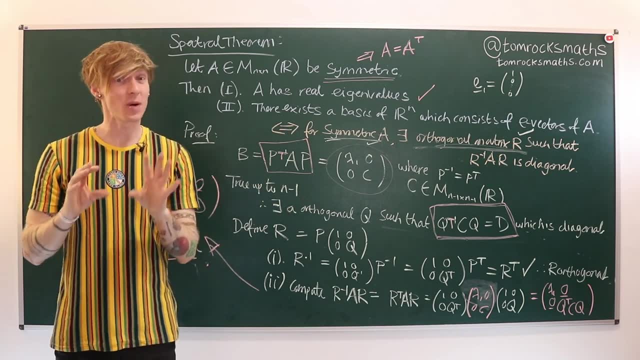 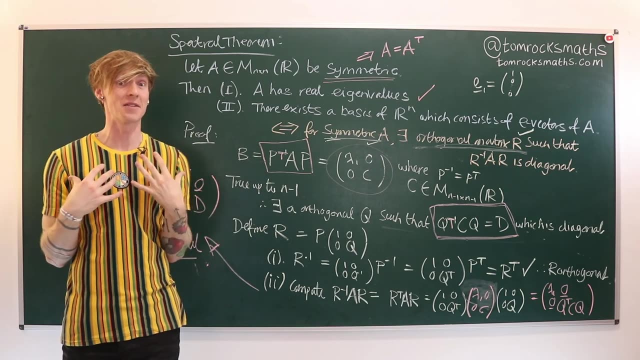 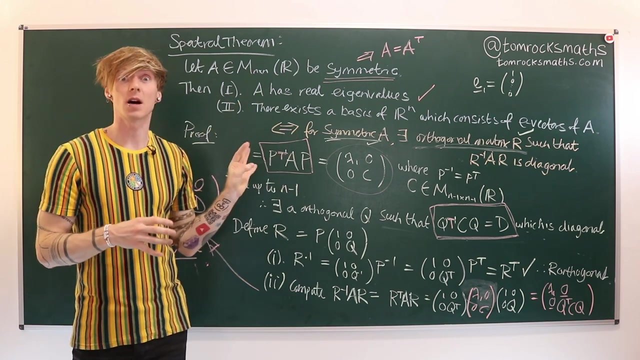 Thing All Put Together Gives Us A Full Proof Of The Spectral Theorem. I Will Just Add A Very Important Point At The End Now. 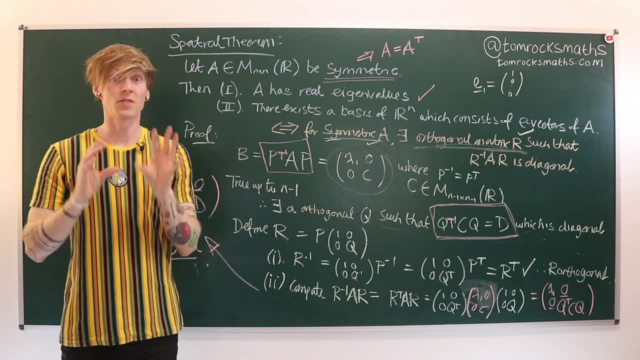 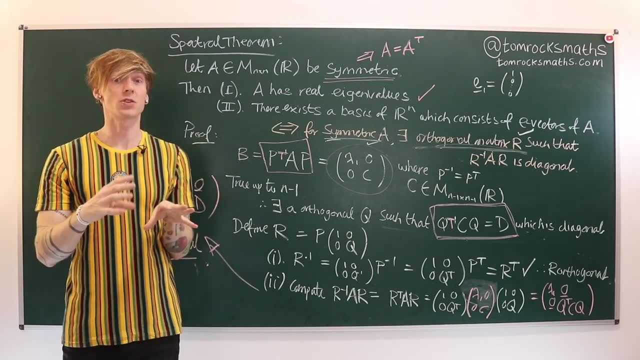 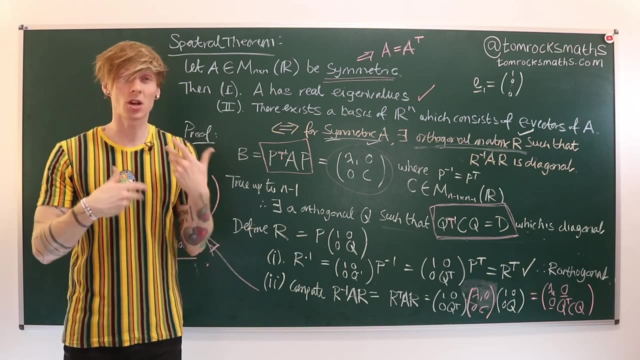 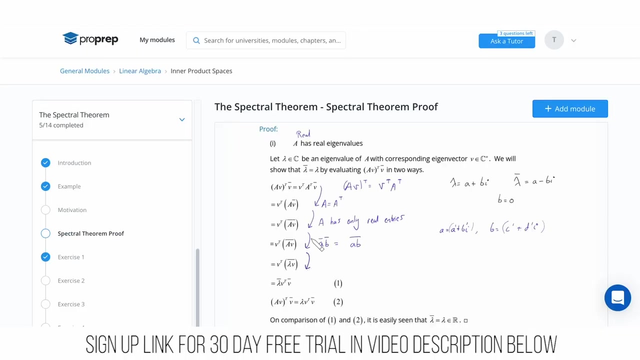 That I Really Do. Recommend, First Of All, Rewatching This Video And Pausing, Working Through Each Step For Yourself To Make Sure You Are Happy. 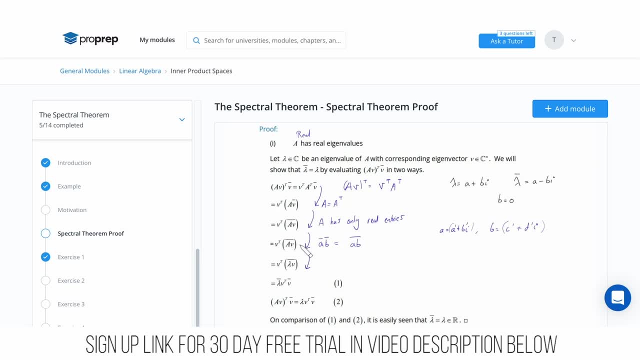 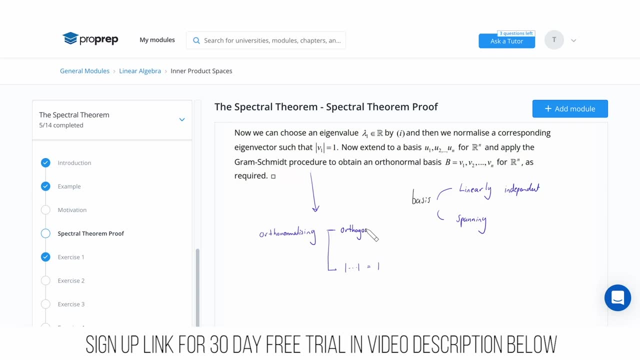 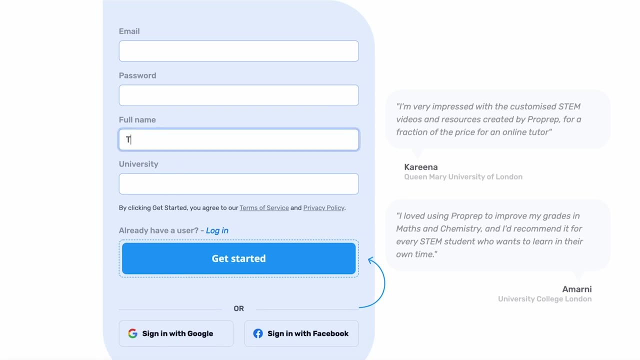 With Each Deduction That's Being In The Description, The Box Right Below What You're Watching Now. So Do Check That Out And Remember You. 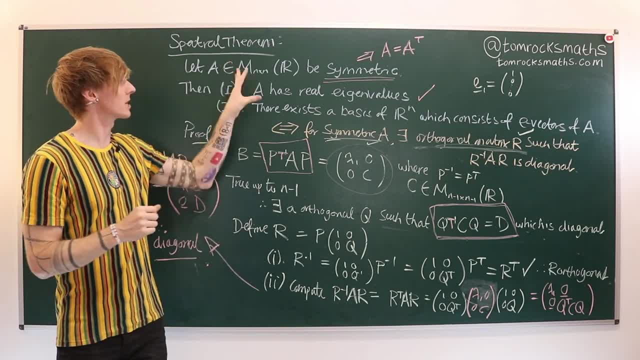 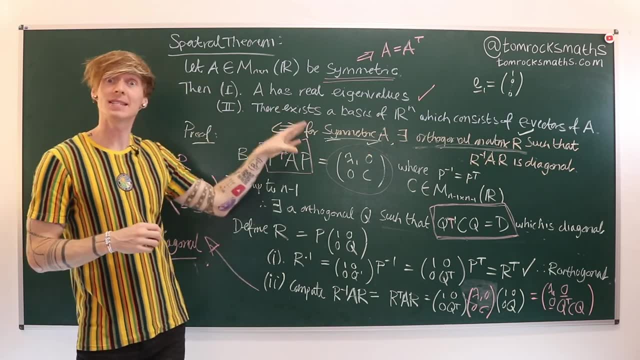 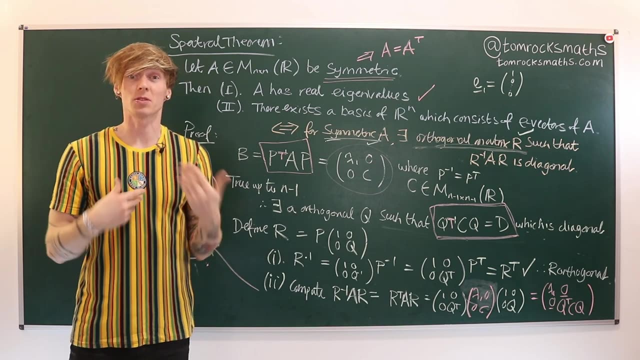 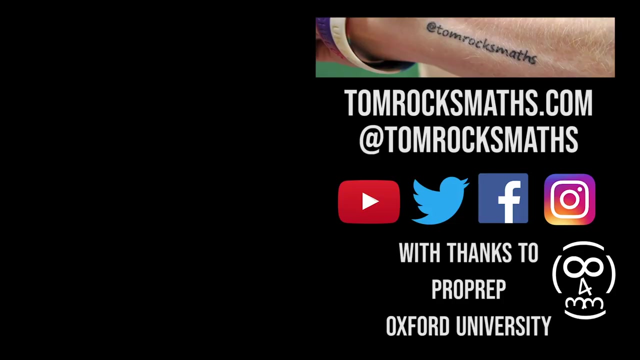 Can Click On The Link To Sign Up For A Basis Of Eigen Vectors. Thank You, As Always, For Watching. Please Do Remember To Subscribe. 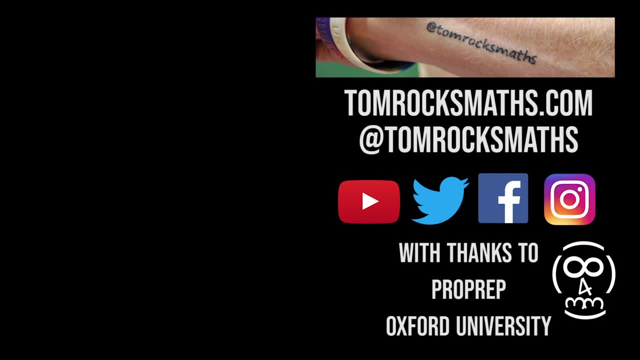 If You've Enjoyed The Video And I'll See You All Soon- Take Care.